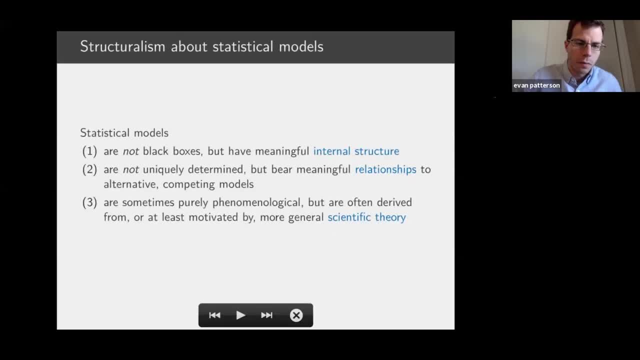 So I'm sorry, Evan, you're muted. Okay, good now. Okay, yeah. So the general viewpoint for this is to try to understand statistical models and structuralist kind of way. So this means that statistical models are not black boxes, but they have meaningful internal structure, which is often of interest. 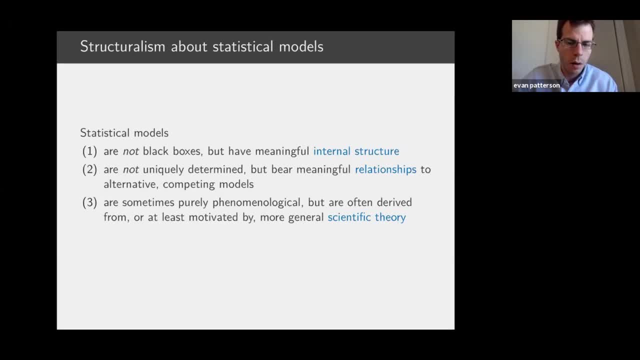 in particular, applications and sciences. Another aspect of models is that, contrary to the idea that you might get from like a introductory textbook, like, they're not actually uniquely determined by like the kind of data that you have. They're often different, competing models and those models bear meaningful relationships to each other. 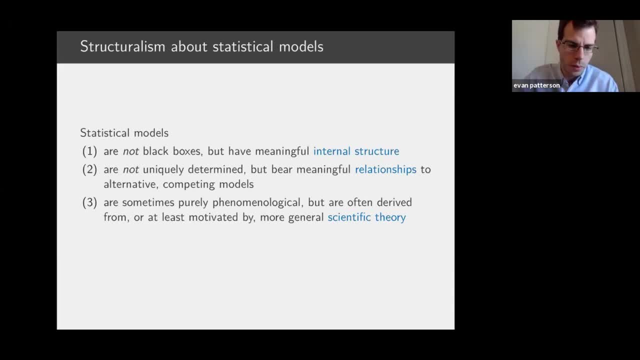 And finally, although sometimes models are purely phenomenological, that is, they're just sort of written down because they seem to fit the data, They're often motivated by, at least, or maybe even more strongly related to, a more general theory that one's trying to investigate. Okay, so, 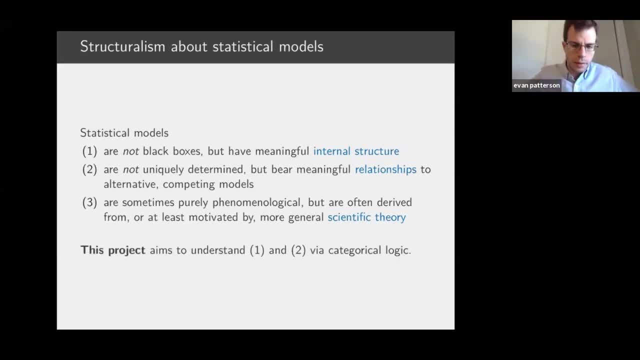 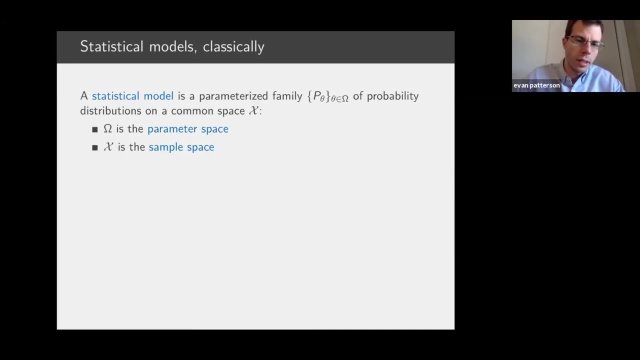 the goal of this project is to understand that. the first two points, at least by categorical logic. the third not so much. Maybe I'll say a little bit about it at the end. Okay, so so in a classical sense, a statistical model is usually defined to be a parameterized family. 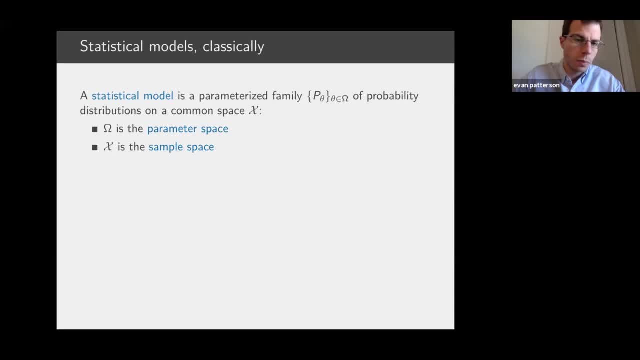 of probability distributions on a common space, x, which is called the sample space. So for every point in your parameter space you get a distribution on the sample space, And then you know. we think of a model like this as being a data generating mechanism. So there's some unknown. 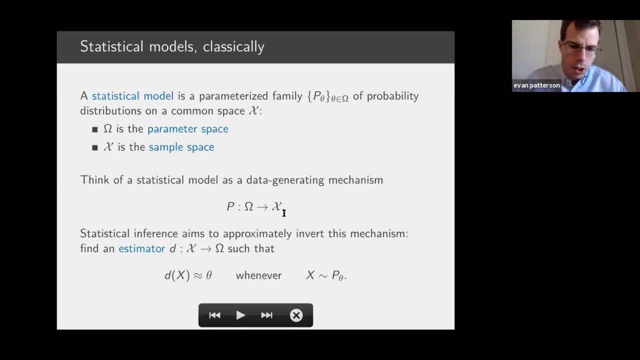 parameter, and then we think of a model like this as being a data generating mechanism. So there's some unknown parameter which defines a probability distribution that generates data and then, given a sample of that data, the aim of statistical inference is to invert, at least approximately almost always. 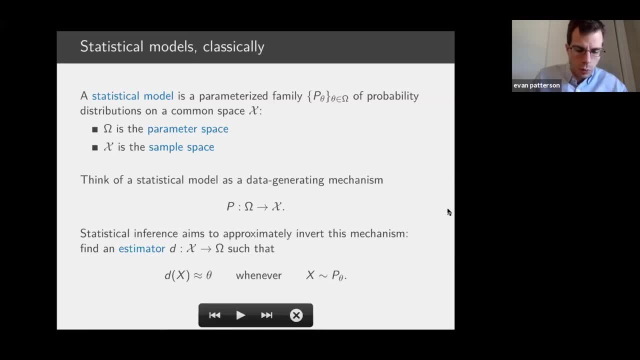 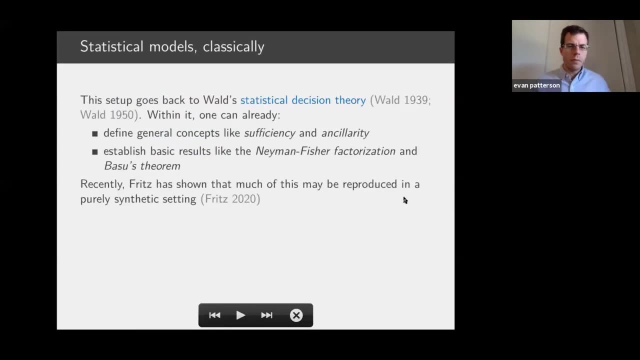 approximately this mechanism. Okay, so that's what statistics is all about in a nutshell, And this simple formalism that I just introduced. it goes back, at least, to Abraham Wald, so to his statistical decision theory, which was the early framework to sort of formalize theoretical statistics in kind of a general way. 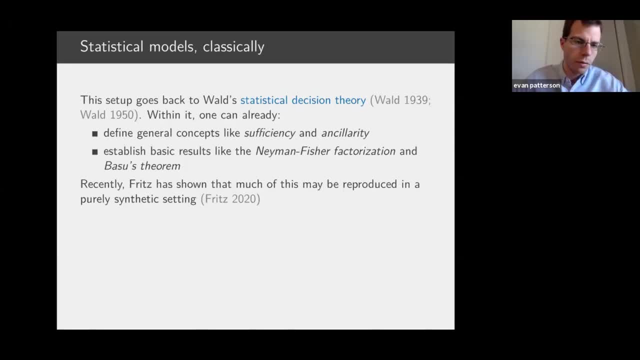 And within this formalism, you can already do a fair number of things. You can, you know, even though this definition of a statistical model is very minimal. you can already define concepts like sufficiency and ancillarity and establish certain basic generic results such as, like the Neyman-Fisher factorization criterion or Basu's theorem. 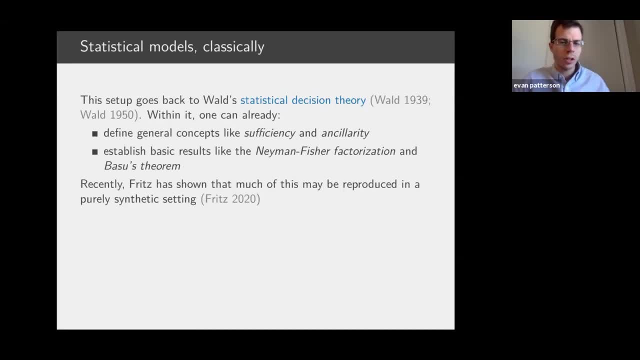 And recently Tobias Frist has shown that actually a lot of these definitions and abstract results can be reproduced in a purely synthetic setting of Markov kernel. so Markov categories- So we'll say more about those later- And that's quite remarkable. Nevertheless, this classical definition, 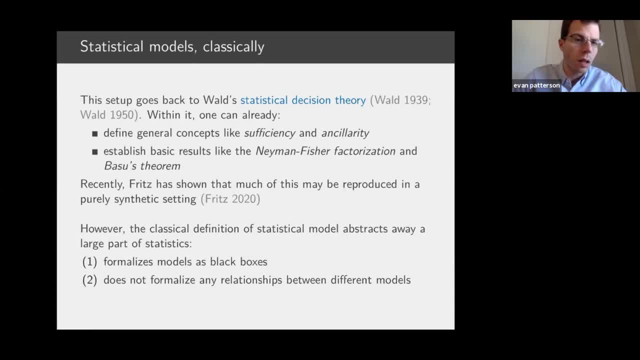 of statistics is abstracting away from a lot of essential things. So, by the way that this family probability distributions is defined as having no further structure, that's essentially treating the model as a black box, at least as far as the mathematical formalism is concerned. And, moreover, 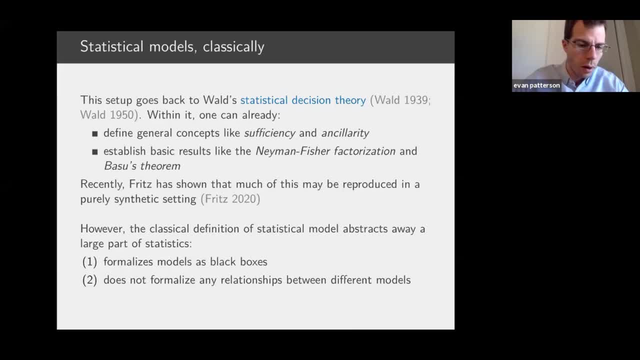 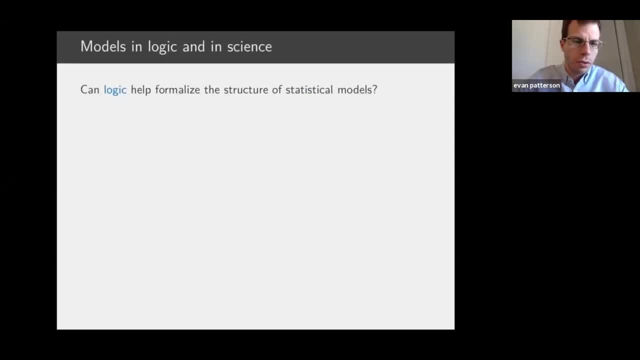 it doesn't really provide any guidance at all on how one might model or formalize relationships between different models. Okay, so if we'd like to do those things, I think it's natural to ask whether logic can help in formalizing the structure, And that's certainly not a new idea to try to. 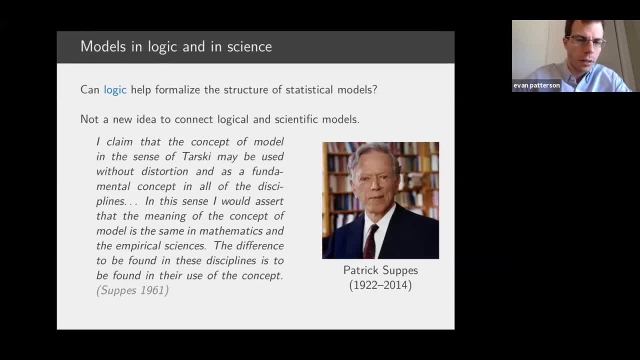 understand how mathematical logic is connected to scientific models in science, or even statistical models specifically. So here's Patrick Supp's writing in 1961. He says: I claim that the concept of model in the sense of Tarski may be used without distortion. but it's not. 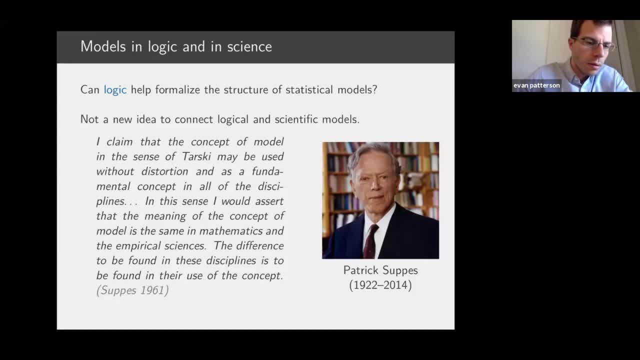 It has a fundamental concept in all of the disciplines. In this sense, I would assert that the concept of the model is the same in mathematics and the empirical sciences. The difference to be found in these disciplines is to be found in their use of the concept. So he's saying here that the 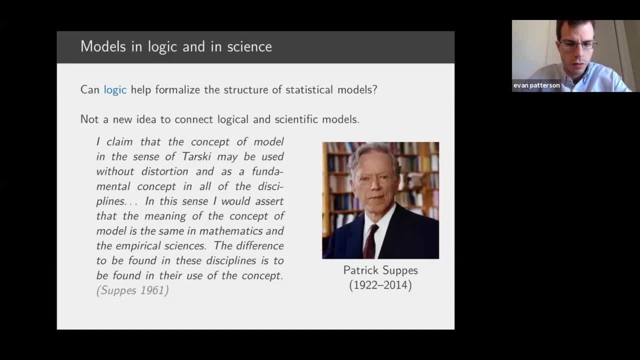 notion of model that Tarski introduced, and which is fundamental in mathematical logic, can also be implied to empirical models, with the understanding that, however, the way that those models are used or derived is different, but the underlying concepts are closely aligned. So this led to a viewpoint mainly within the philosophy of science. 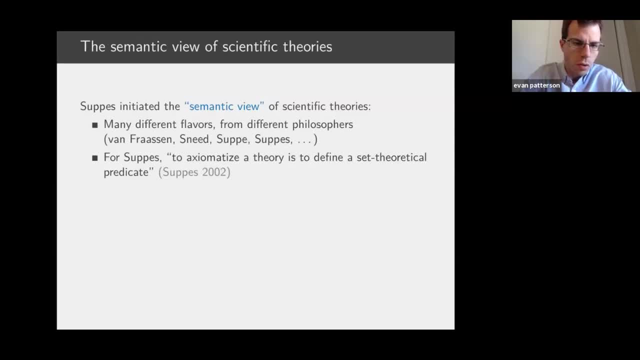 called the semantic view of scientific theories, And there are a lot of different flavors of it. In Supp's flavor the idea is to axiomatize a scientific theory using a set theoretical predicate. But from the viewpoint of this work there are 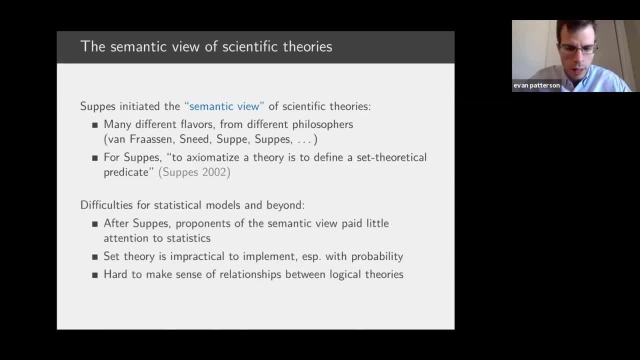 a number of difficulties with this. First of all, despite the fact that Supp's was, among other things, a statistician, subsequent workers on this viewpoint did not really pay a lot of attention to statistics, So that aspect of it was never really developed. 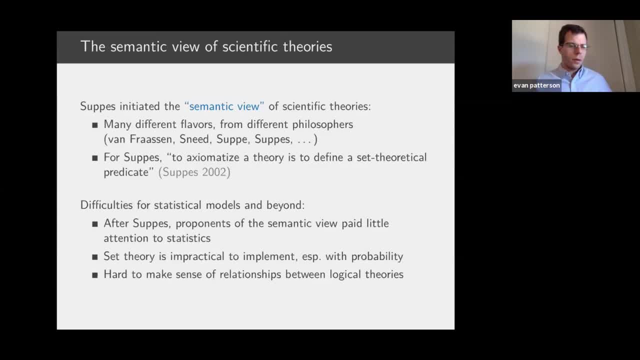 The working sort of purely in set theory like Supp's did is sort of awkward because it requires people to encode into set theory all the parts of real analysis and probability that you need. But I think most importantly that way of thinking about things does not directly provide a lot of 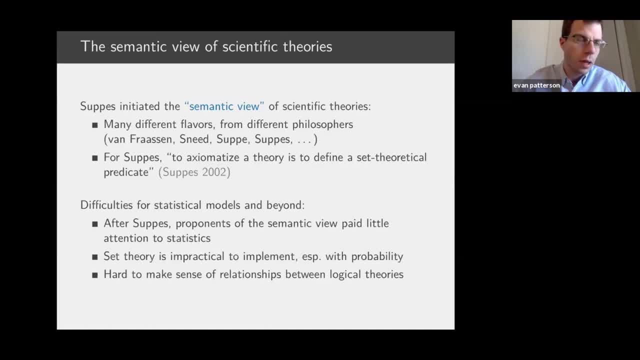 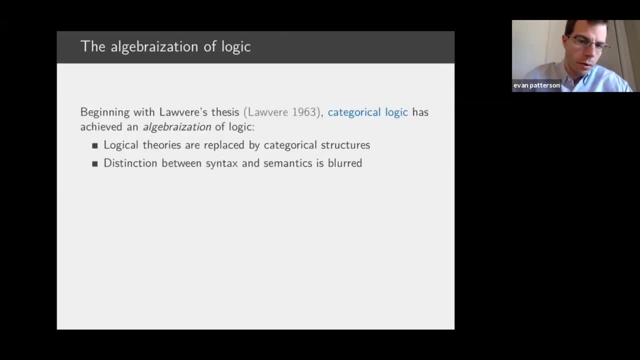 guidance on how to make sense of relationships between different logical theories. And this is where, I think, category theory, specifically categorical logic, starts to come in. So in his seminal PhD thesis in 1963, Lavier achieved a so-called algebraization of logic. And so what? 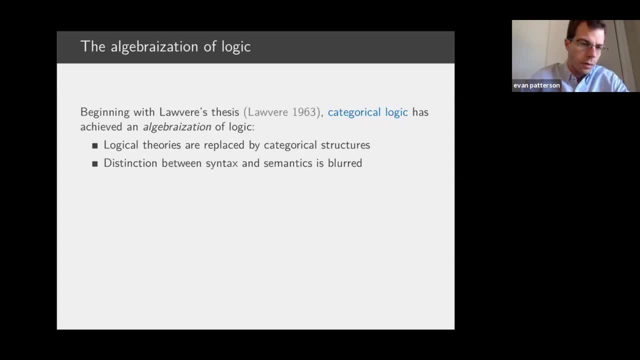 happens in this setup is that logical theories, traditionally conceived of as purely syntactical objects, are replaced by certain kinds of categories And, as a result of this, the classic distinction between syntax and semantics is blurred. This change in viewpoint has a lot of important consequences. 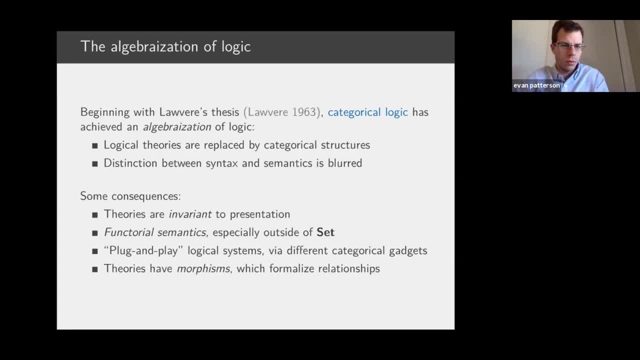 I think, all of which will be irrelevant to us. So, from this viewpoint, logical theories become they're algebraic objects, so they become invariant to changes in the way that they're presented. The idea of functorial semantics which follows from this makes it really 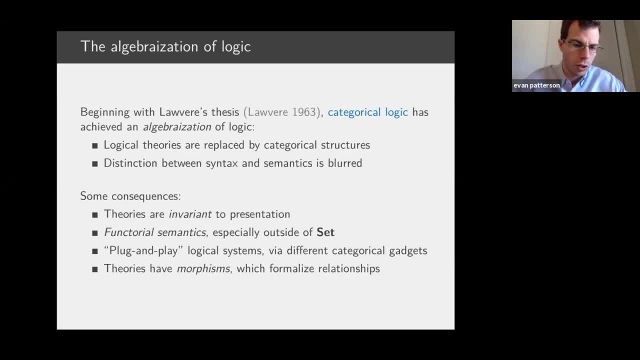 easy to get semantics outside of the traditional setting of sets and functions, which for probabilistic settings is really important. So we're not going to be working in the category of sets and functions, we'll be working in the category of Markov kernels. It also has sort of 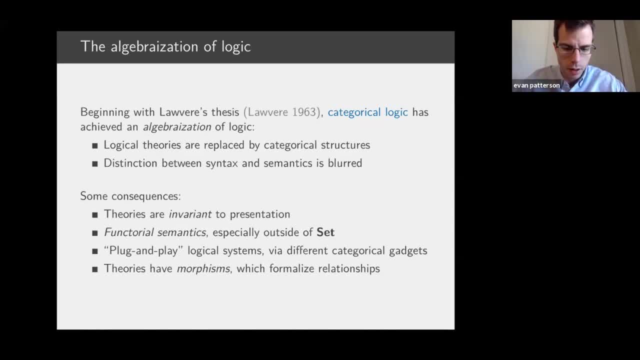 a plug and play aspect right. So category theory provides lots of different algebraic gadgets and it's sort of easy to assemble these together into custom or unorthodox logical systems, And we'll we'll exploit that. And finally, once you've turned logical theories into algebraic structures, 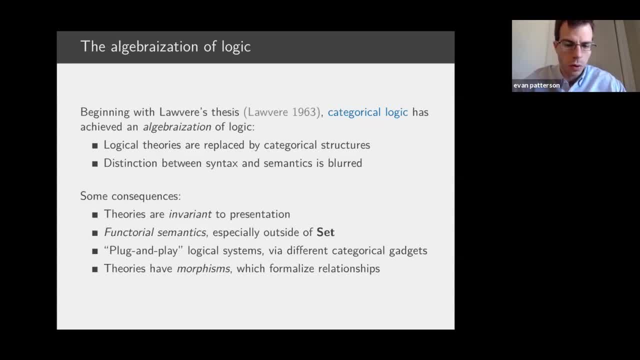 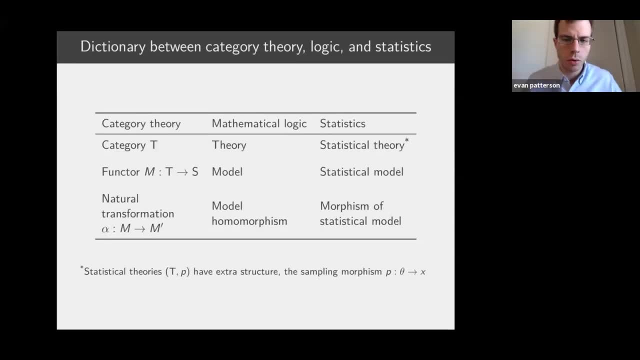 well then, they have morphisms, just like any other kind of algebraic structure, and we'll use those to formalize the relationships between statistical theories and models. Okay so, so here is sort of an overview of how this picture sees statistics as fitting in with categorical logic. So, 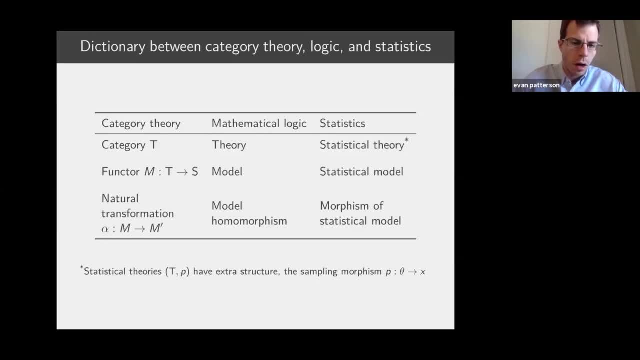 statistical theories are going to be a certain kind of category, and then functors out of those theories will be statistical models and finally, natural transformations between those will be morphisms- statistical models. Okay, so this is extending sort of the famous dictionary of categorical logic. 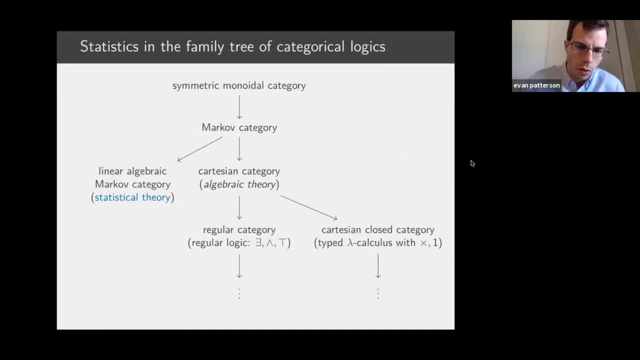 Okay. so to try to put this in in context a little more so, traditionally categorical logic begins, as it did in Lavier's work, with the study of algebraic theories. So these correspond to Cartesian categories, or finite products categories, And a lot, of, an enormous amount of work in 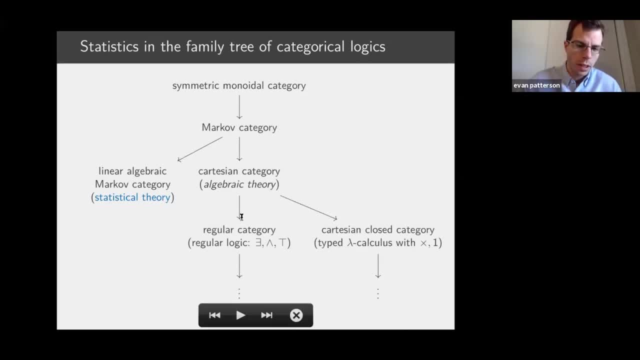 categorical logic has come from extending these kinds of theories to richer logical and type theoretic settings. So in one direction you can start developing regular logic and then coherent logic and eventually reach topos and so forth. In another direction you can start to 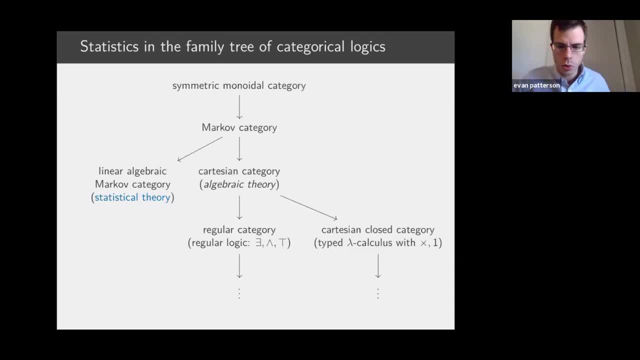 develop the type lambda calculus which corresponds to Cartesian closed categories, and there's a whole line of work in that direction as well. So in this work we're sort of branching off into a different direction of the of the family tree. So we're going to be working instead. 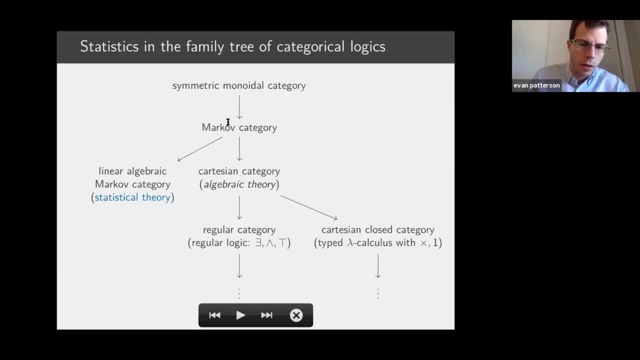 of with Cartesian categories, with Markov categories. So these are actually weaker than than Cartesian categories because they allow non-determinism. And then we're also going to be attaching to that some additional linear algebraic structure to capture in order to be able to talk. 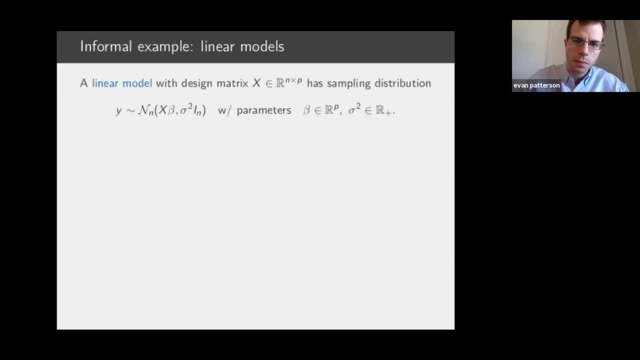 about a lot of commonly used statistical models. Okay, so let me give an informal example of this, which I'll return to to later. So a linear model would ordinarily be defined in this way. You know, say that, given a design matrix which has n rows and p columns, where n is the number of 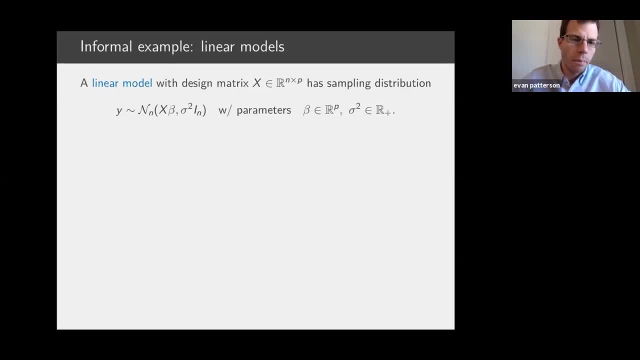 observation p is the predictors. a linear model would be a normal sample drawn with mean of the design matrix, times some unknown coefficients or parameters, beta, and then having a and then having a spherical covariance determined by this variance parameter. Okay, and so what we'll say is that there's a, there's a. 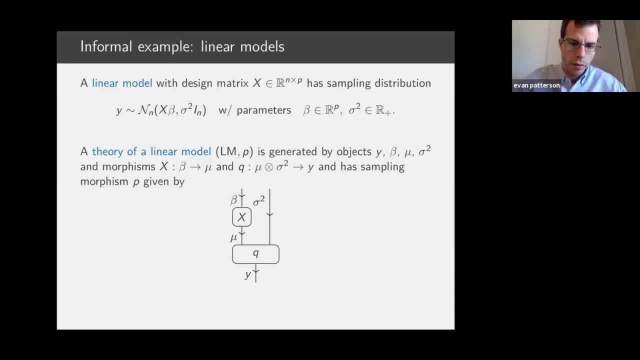 actually a theory behind this, a theory in the sense of categorical logic, And it is so. it's a certain kind of category, and it's generated by some objects and some morphisms, And then, moreover, there's also a stipulated sampling morphism which looks like this: So that's. 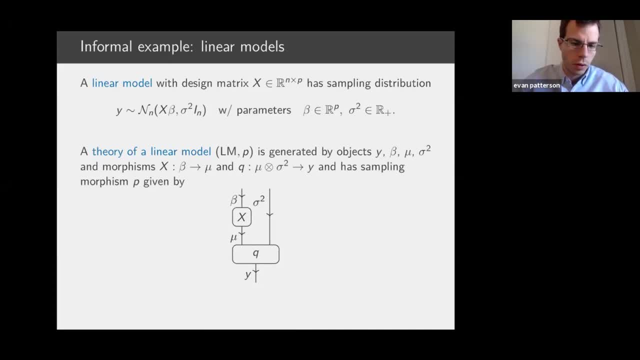 sort of capturing the sampling distribution in terms of the generators, And we can see the design matrix x here in this simple example, as well as q, which represents the random component of the model. This would be the typically the the isotropic Gaussian. 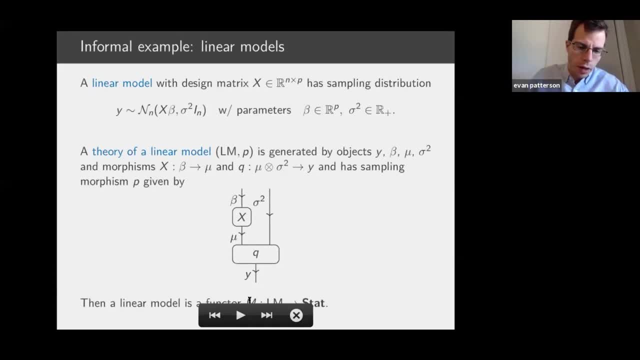 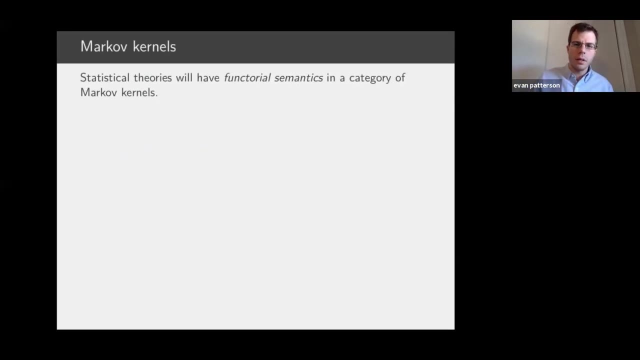 Okay, and then, having said that, a linear model then becomes a functor. Sorry, that thing is blocking the text. A linear model becomes a functor from this theory into this category stat, of course, markup kernels, which we'll see. Okay, so that is the the introduction, And so now we're going to. 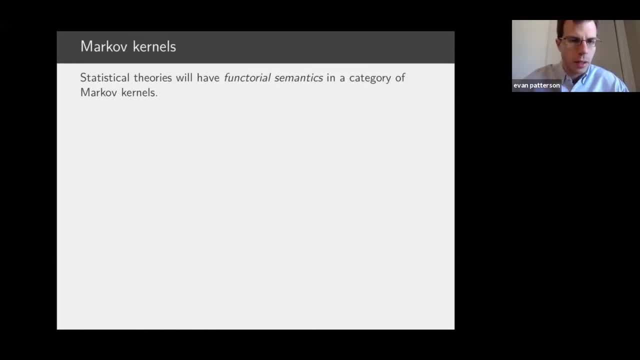 start to to develop some of these ideas in a bit more detail. So sorry, Evan, Yes, I forgot to ask you before. Sorry about that. Do you prefer to be asked questions during your talk, Or will you stop, or at the end? I think at the end is is better for me. I'll try to leave some some time at the end. 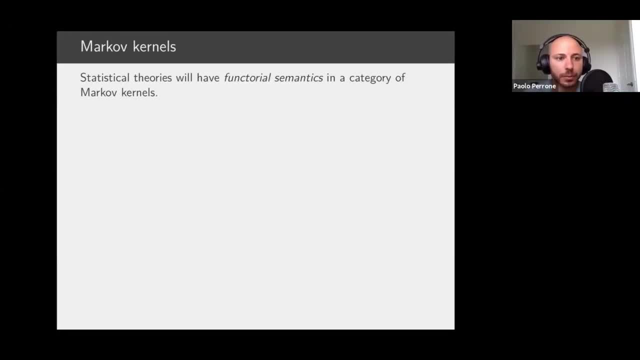 of that, Thanks. Okay, very good, Thank you. So. so, as I've said, statistical theories will have functorial semantics in a category of of Markov kernels, So let's review what those are. So, formally speaking, a Markov kernel- excuse me- is a function from a measurable space into the space. 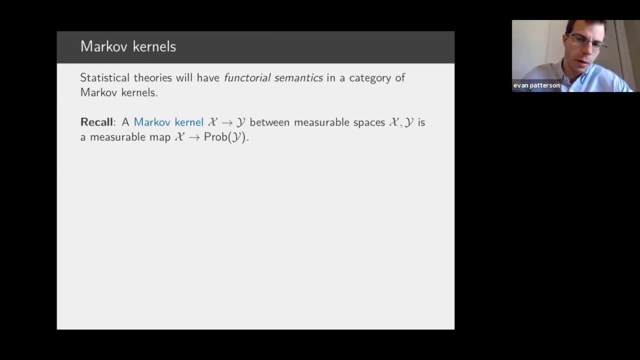 of probability distributions on another measurable space And it has the intuitive interpretation is just being a probabilistic function. So to every point in the domain you assign not just a, a single point in the codomain, but actually a probability distribution over the codomain. 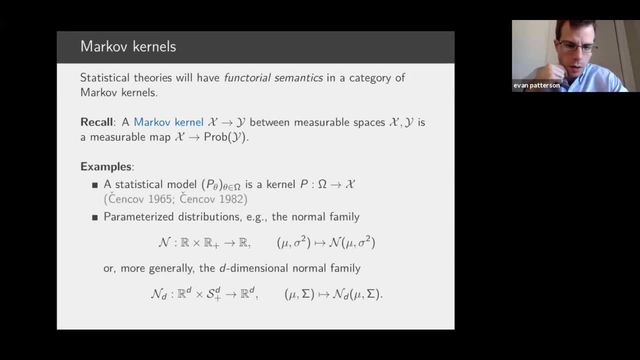 And so some examples of Markov kernels that are very relevant to this work. Well, in the first instance, a statistical model in the classical sense, by just changing our viewpoint a little bit, can be seen as a kernel, a Markov kernel, from the 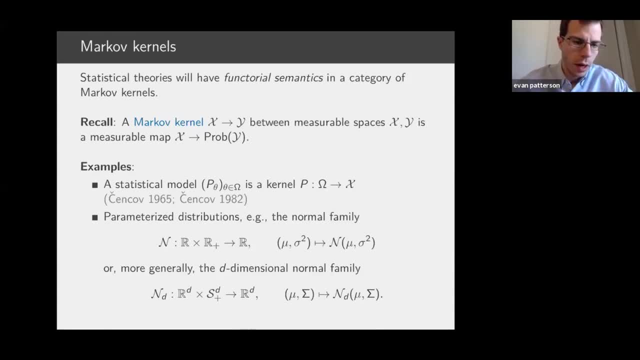 methodazzation of a parameter space into the sample space, And I think that the Tsentrov was the the first to really take this viewpoint seriously in and and in trying to develop a categorical formalism around this. That work actually goes back quite a long ways, In addition. 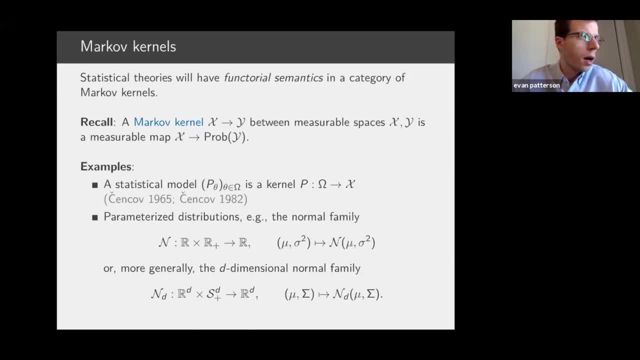 essentially any parameterized family of probability distributions. instead of thinking them as thinking of them as being a set of distributions, we can think of them as not being a whole set of thingsologically, think of them as being a single object, this Markov kernel. 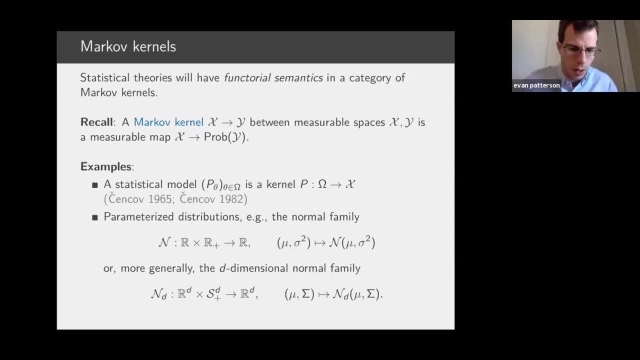 So, for example, the normal distribution can be seen as a the normal family, rather can be seen as a kernel which maps a mean and a variance to the normal distribution, having that mean and variance, And similarly for the higher dimensional normal distributions and essentially any other parametric family that you like. 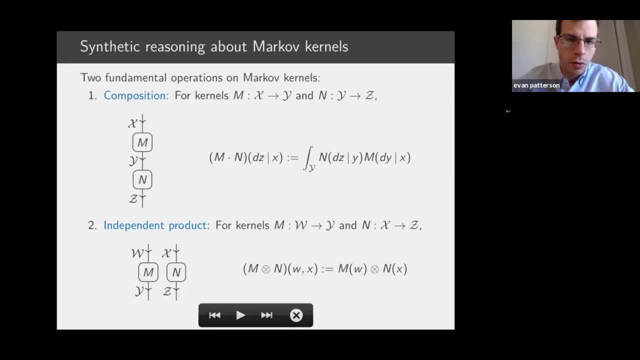 Okay, so there are two fundamental things that you can do with Markov kernels, basic building blocks, So you can compose them, which has a natural probabilistic interpretation, But we can think of this as just generalizing composition of functions. And then there's also the independent product. 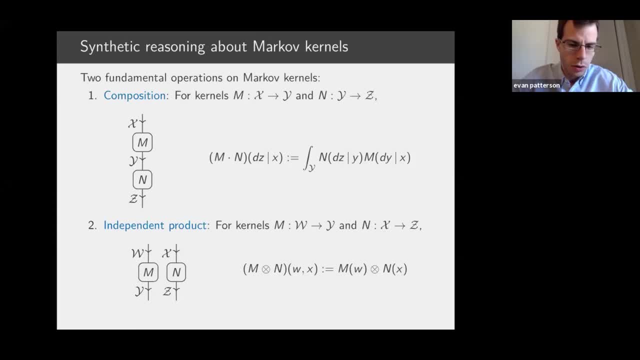 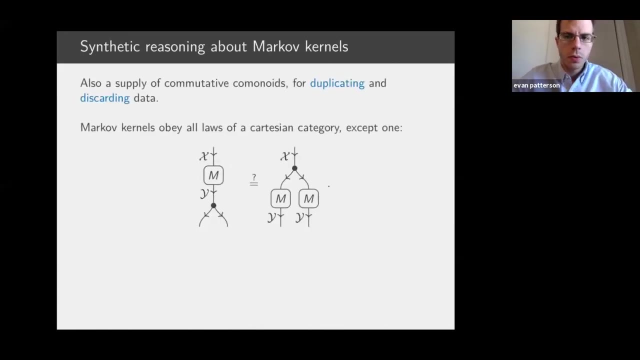 So where given to Markov kernels, you get the independent product by at every pair of points you take the product distribution in the co-domains. Okay, so these two things give the category of Markov kernels the structure of a symmetric, monodal category. 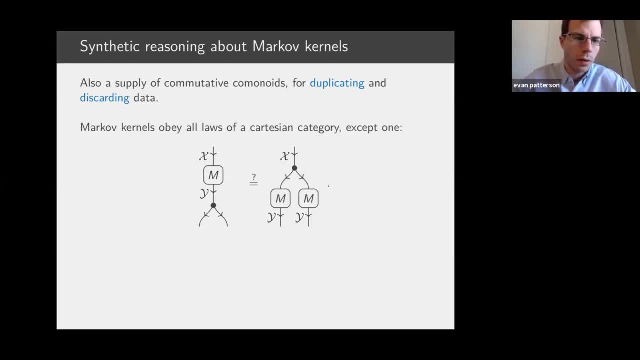 There's also a supply of commutative commonoids which allow data to be duplicated or discarded. And having set this up, one sees that this category obeys all the laws of the Cartesian category except the one. So the law of a Cartesian category. 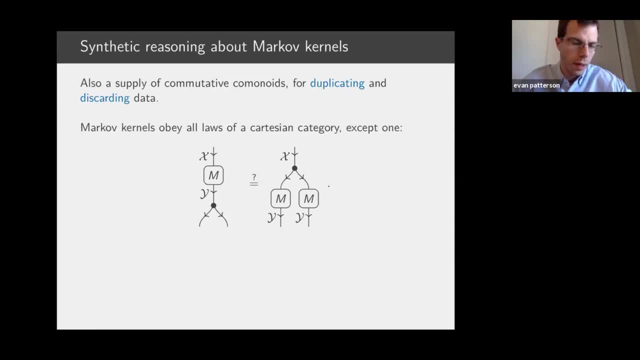 that basically, morphisms preserve, copying does not hold, And that is a reflection of non-determinism as essential property of this category. So in fact, you could show that if your Markov kernels are reasonably well behaved, then this equation will hold, if and only if. fine construct of n crochet within the assume nature andください, counter Menybib and object. we can show your Marco, kernels are usually well behaved. then this equation will hold. it's an only if콰tion of n, corner, Y25, nZ, and you calculate the boundary, whether they produce them asquittal, so at the observation will hold theshaped PBC given by Jesus by counting dataammed by two relationships, the usingovers and exponents, and going up and creating the decision behind. 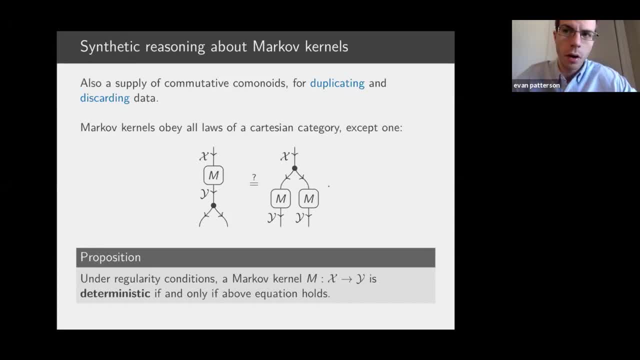 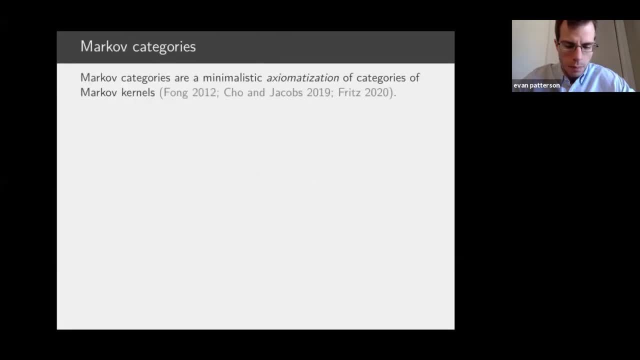 if they're deterministic, meaning that they essentially are just functions, And so this viewpoint leads to the idea of a Markov category. So I believe Fritz coined this term fairly recently, but the idea goes back longer than that. It's been studied by a number of people under different names, And so a Markov. 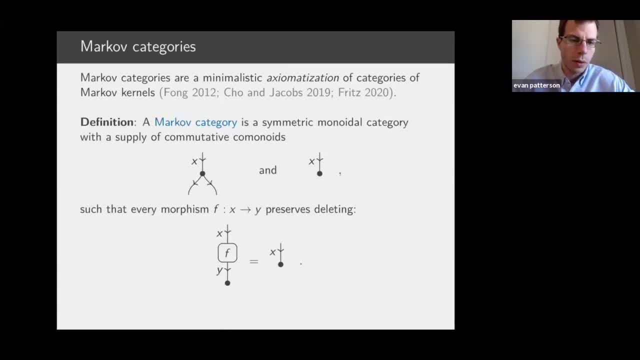 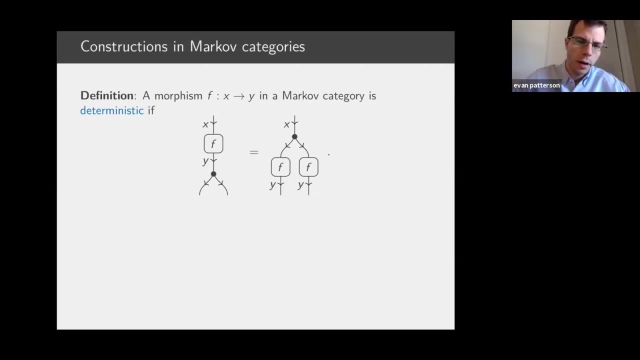 category is defined to be a symmetric monoidal category with a supply of the commutative combinoids such that every morphism preserves the deleting operation but, as we've seen, not necessarily copying, And you can express a number of different probabilistic constructions within a 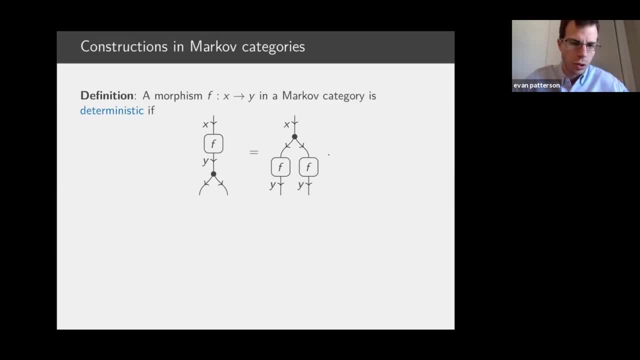 Markov category. So, having seen this proposition, it's natural to turn this into a Markov category. So, having seen this proposition, it's natural to turn that around into a definition and say that a morphism in a Markov category is deterministic if it preserves copying. And in addition to that one can: 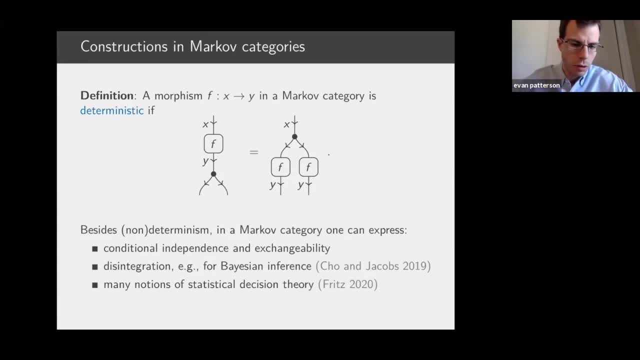 express a fair amount of other things, So different notions of conditional independence and exchangeability. You can express the notion of disintegration, which is essentially a form of Bayes rule, so very important in Bayesian inference, And, as I mentioned a bit earlier, you can actually formulate a number of notions of 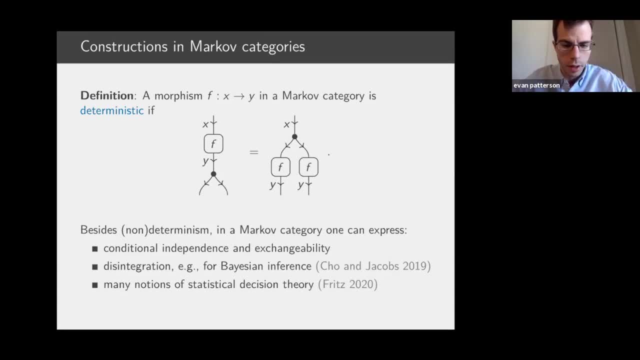 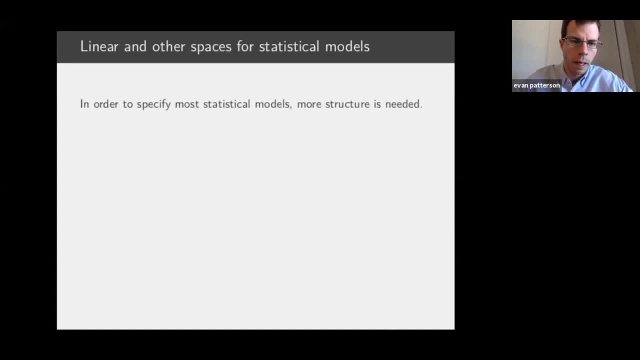 statistical decision theory, such as sufficiency, ancillarity and so on, within this framework. So, despite its minimalism, it is surprisingly useful Nevertheless, if we want to actually specify a concrete statistical model of the sort that not sort of like a very general class of models, but a more concrete one, usually we need some more. 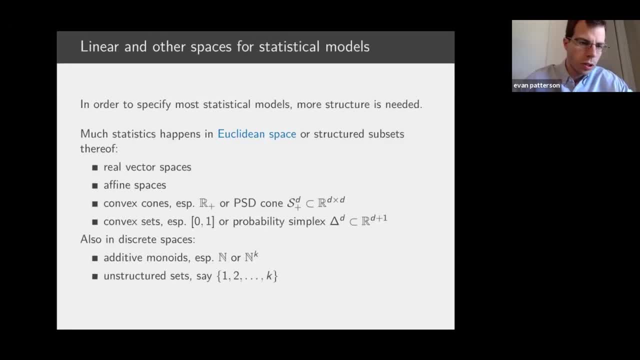 structure than this. So most of classic applied statistics is happening in Euclidean space or in certain structured subsets of that, So in affine subspaces, in convex cones. so most importantly the non-negative reals, or it's the relevant generalization in higher dimensions. 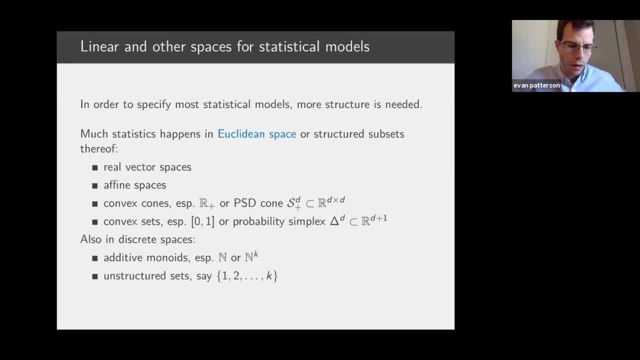 here is the positive semi-definite cone. That's where variance matrices live, Or in convex sets. so the unit interval or the higher dimensions of the simplex. This is where the parameters of the multinomial distribution live, And then also some discrete spaces. 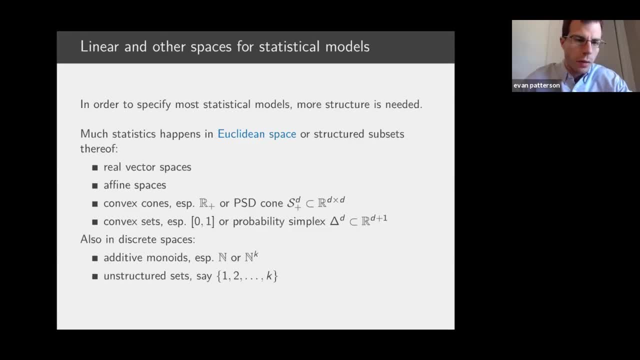 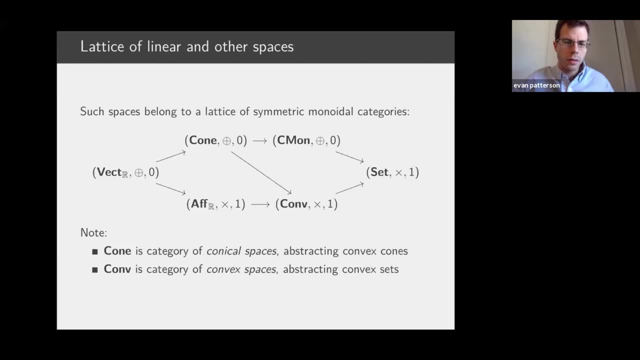 particularly the natural numbers, so that you can count things- So basic stuff that we need in order to set up a lot of models, And these different spaces can be seen to form basically a lattice, where sort of the most structured spaces are vector spaces and the least structured ones are 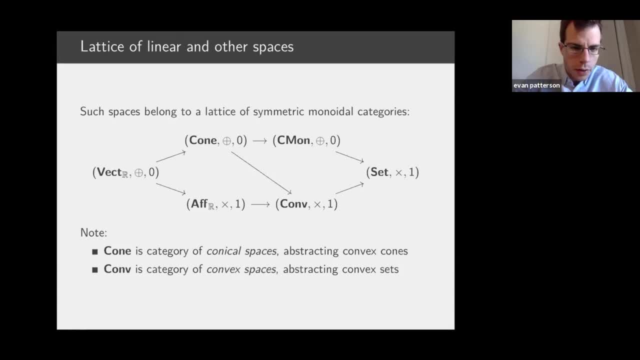 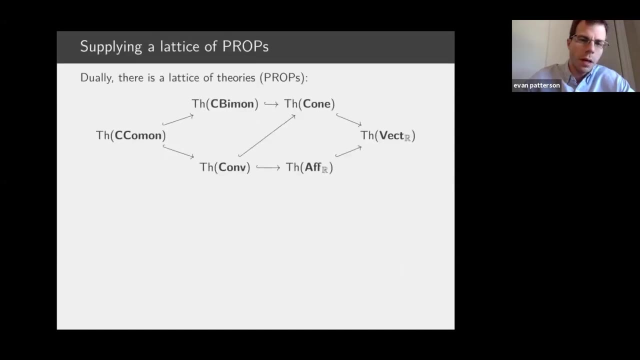 sets, And then there are these intermediate spaces, where that the affine spaces, the conical spaces, the convex spaces and the monoids live Okay, and so this can be turned around. So we want to try to formalize some of these properties, some of these structures and some of these. 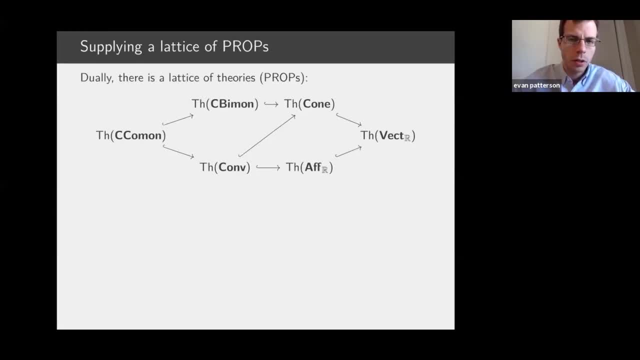 spaces in a purely algebraic way. Okay, so what we're going to do is sort of turn the arrows around to get and see that the theories- which in this case are props- corresponding to these different structures form this dual lattice. And so we will, with this example in mind, 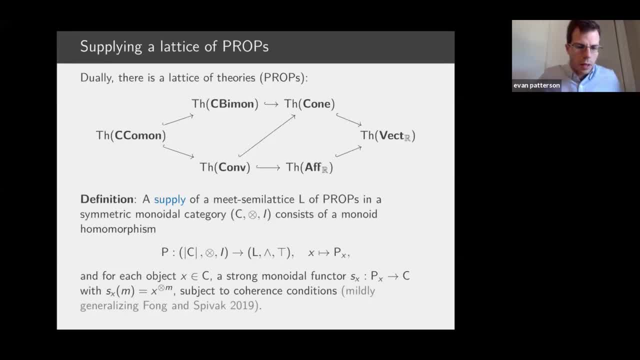 we're going to generalize slightly the notion of supply that Fong and Spivak introduced to allow supplying a lattice of props in a symmetric, mononomic category as opposed to just one. So we'll say that a supply of a semi-lattice like this in a symmetric 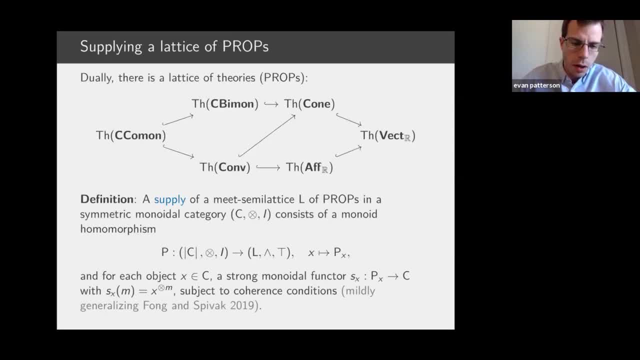 mononomic category consists of monoid homomorphism on the objects of C into this lattice where the. so basically, what we're saying here is that when you take the product of two, the mineral product of two objects, then the structure that they get should be the join of. 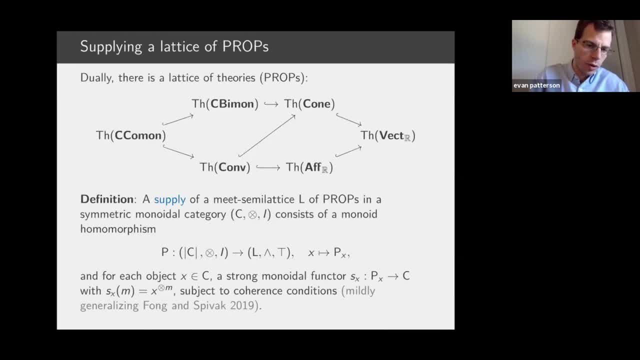 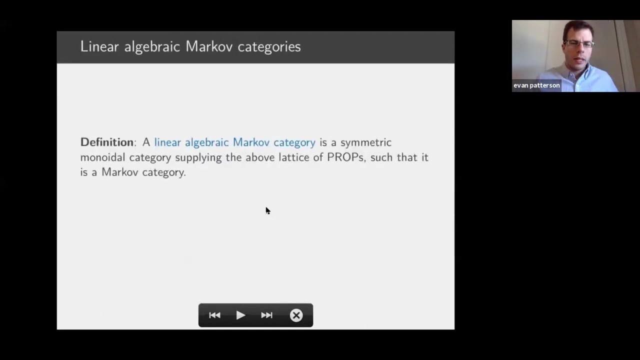 the structure of those two objects right. So, for example, like, if you take the product of like an affine space with a conical one, you should get a convex space. So that's just formalizing that idea And having set that up, 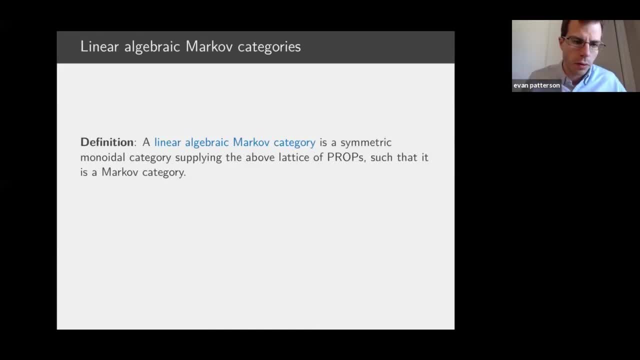 we will say that a linear algebraic Markov category is an SMC, that's supplying this lattice of props in such a way that it's a Markov category. So this is a way of attaching this extra linear algebraic structure to it And basically, like any other kind of 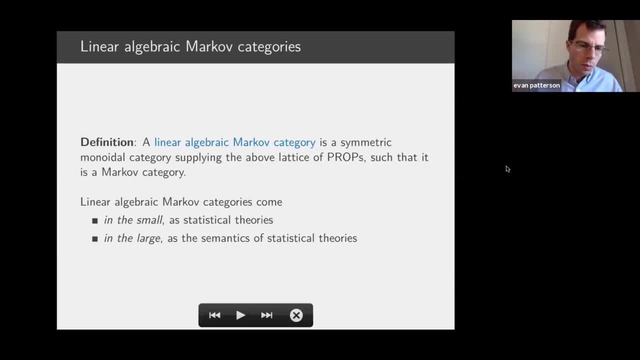 category. they, these categories, come in the small, so as small categories, and these will be the better part of statistical theories- And they also come in the large, and that's going to play the role of semantics in order to define statistical models. So we'll- let's start with. 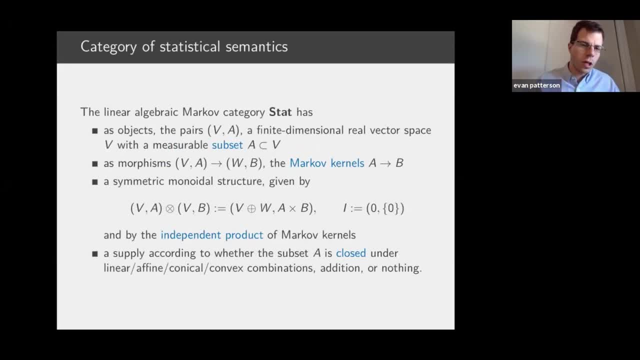 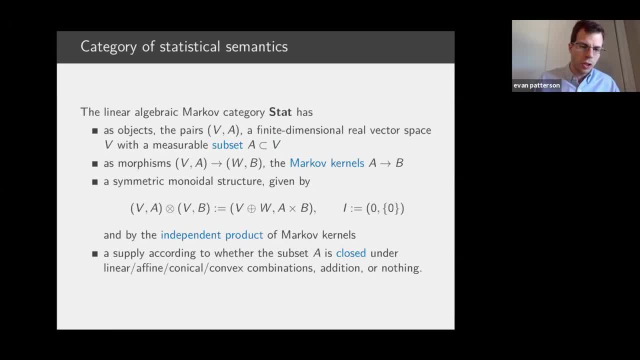 a very simple way to do to do it that that just uses an ambient vector space structure, although there there are other ways. So here we're gonna. in this Markov category stat, we're going to say that the objects are pairs of finite dimensional real vector spaces together. 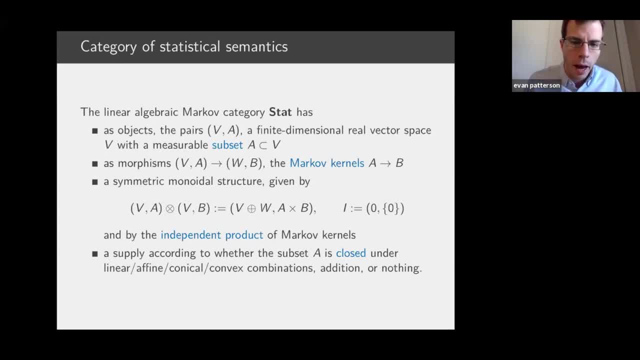 with a measurable subset of that, And then the morphisms are just going to be the Markov kernels between the second part, between those subsets, and having done that we can define a symmetric monoidal structure. on objects will be the Cartesian, the set, theoretic Cartesian product. 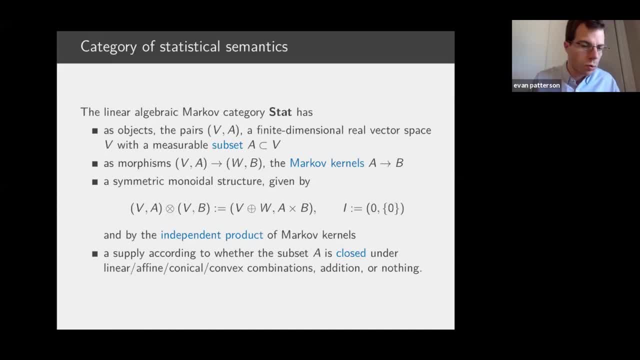 and on morphisms, we're going to take the independent product which we saw earlier, and then it's now pretty easy to define the supply. We'll just say that, you know, a particular object has the structure of a convex space or a affine space or what have you, depending on whether it's 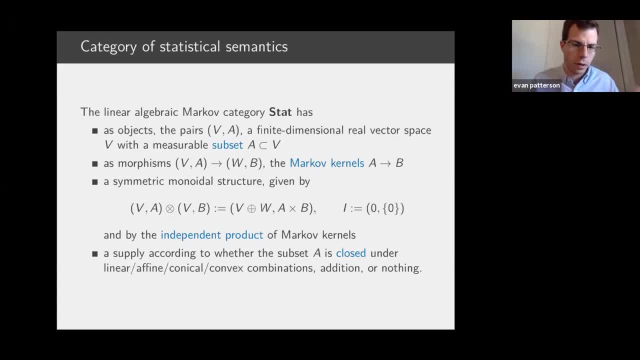 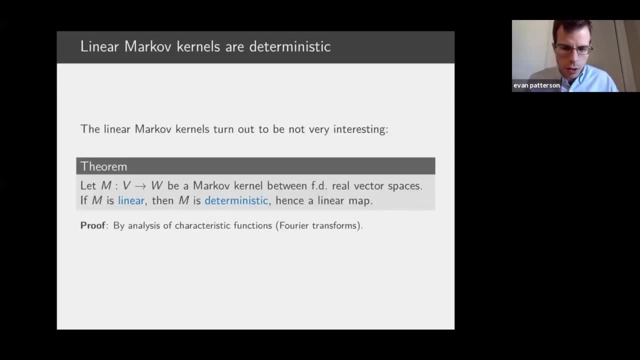 closed under convex combinations or affine combinations or whatever kinds of combinations are appropriate to that structure. Okay, so let's start to look at what some of the morphisms in this category look like. So one thing that should be said, that is that actually the 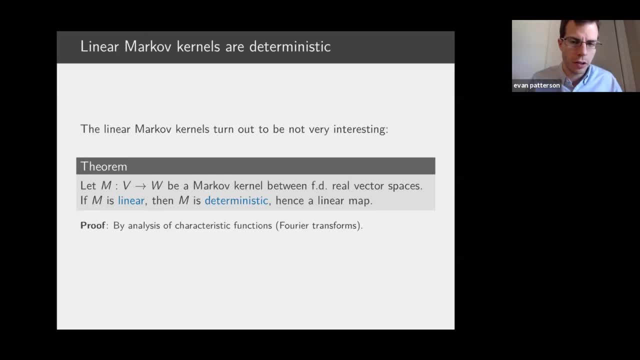 the linear Markov kernels are very uninteresting because it turns out that they have to be determinate So specifically. in other words, if you insist that a Markov kernel between real, finite dimensional, real vector spaces is linear, where you just transplant the normal definition. 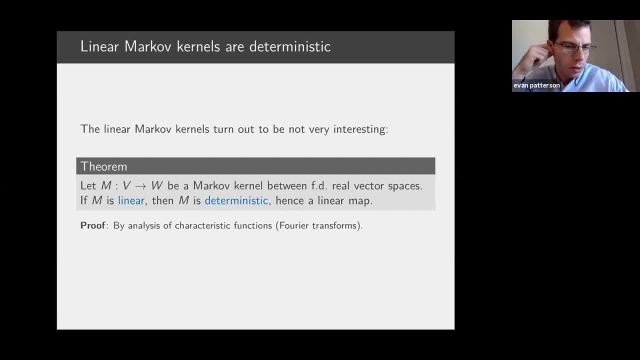 of linearity, then it has to be deterministic, and you can show this by analyzing the characteristic function of this family of distributions. But fortunately there are lots of other interesting kernels that have related properties that look a bit like linearity but are importantly different. 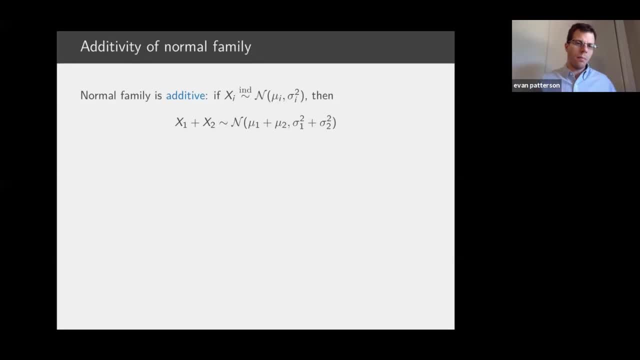 So, for example, the normal family satisfies an additivity property, namely that if you add two independent copies of a normal, you get another normal with the means and variances adding. Okay, so in terms of the morphisms and stat, we can express this equation. 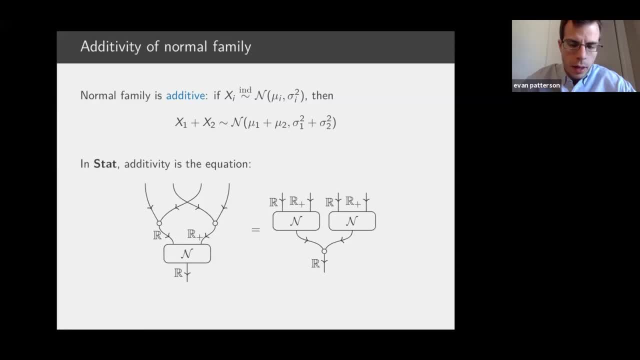 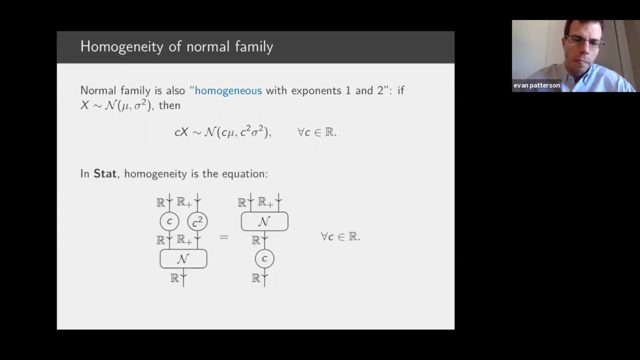 algebraically. So the normal family is homogeneous in a certain sense, namely if you multiply a normal random vector by a constant c, then the mean and variance scale like this, So the mean linearly and the variance quadratically, And this equation becomes this in terms of the morphisms in the category stats. 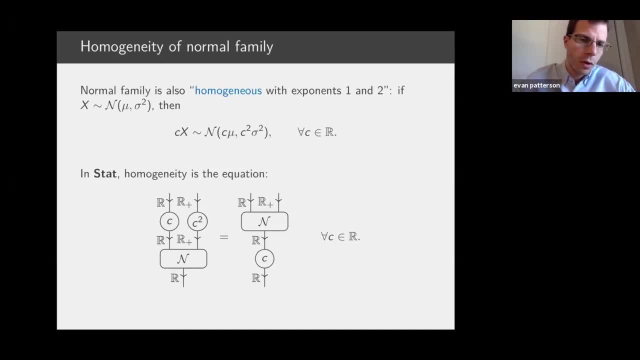 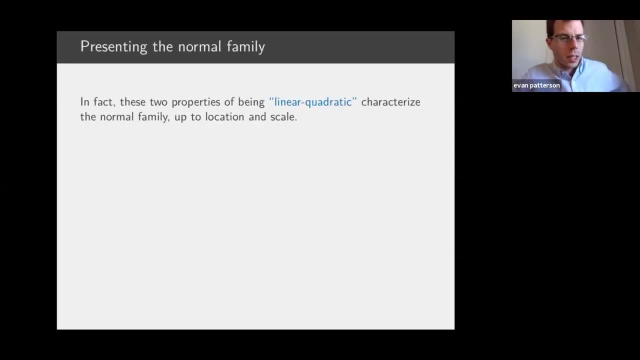 And so it actually turns out. these equations characterize the normal family up to basically linear transformations of location and scale. So, in other words, if I have any linear or quadratic so satisfying these two properties, Markov kernel, where the first component of the domain is Euclidean space, and for 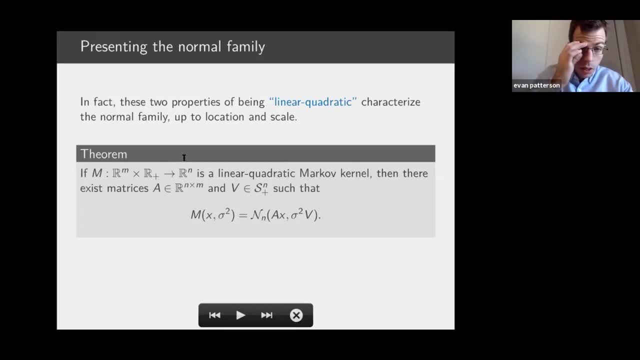 simplicity, we'll just take the second one to be the non-negative reals. then there has to exist a matrix A as well as a fixed covariance matrix B, such that this kernel is the normal family, the n-dimensional normal family, with the mean being multiplied by this matrix A, and then there's the covariance being 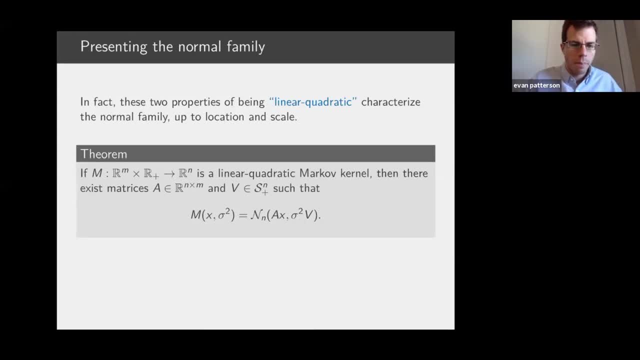 scaled as parameter sigma squared, And this is a little technical, but if you're familiar with the notion of stable families and probability, in the same way you you can present the other symmetric alpha stable families. So the second most important one, besides the normal, is probably the Cauchy. 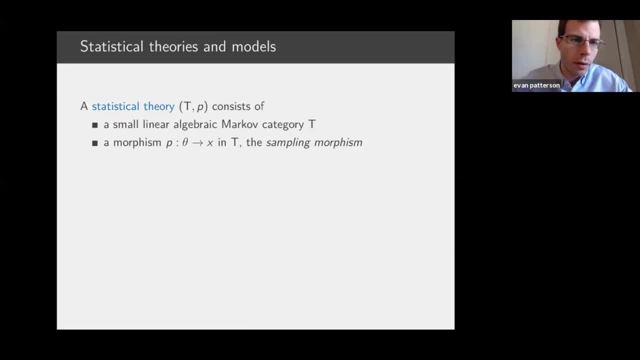 Okay, so that's a little bit of what this category of Markov kernels looks like. So let's move now to talking about statistical theories. So now we're gonna be talking about small linear, algebraic Markov categories, So statistical theory consists of one of those. 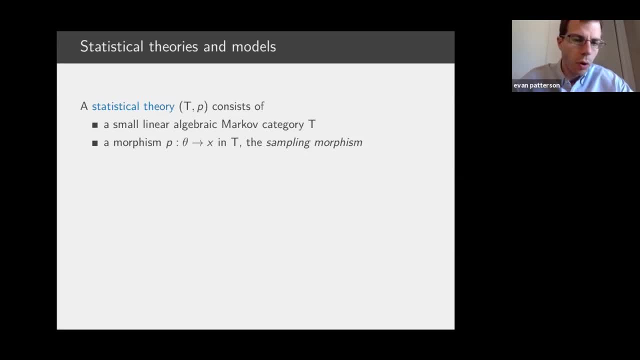 as well as a particular morphism within that theory, which we call the sampling morphism. And having set that up, we can now say simply that a model of a statistical theory or a statistical model is a supply preserving functor from that category in the theory into this category of Markov kernels stat. 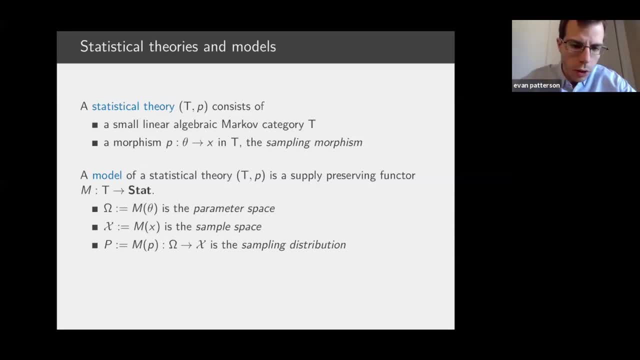 So, in particular, you get a parameter space, you get a sample space and you get a sampling distribution, just like in the classical setting. But now we have this additional structure of the theory coming along which is telling us what different pieces are being assembled to make that sampling distribution. 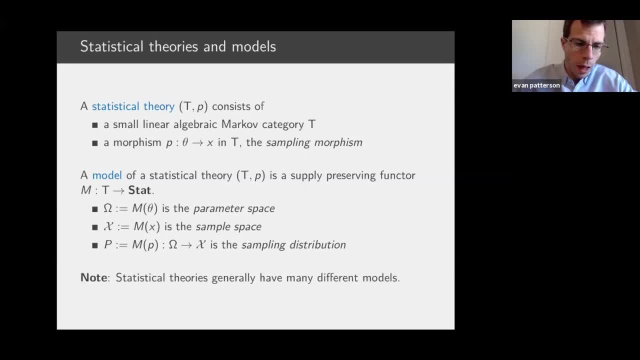 So we'll see some examples For that. I should note that, just as in traditional logic, it's typical that a single theory will have many different models, and that's useful because that allows us to. it's one of the ways in which we can say how different models are related to each. 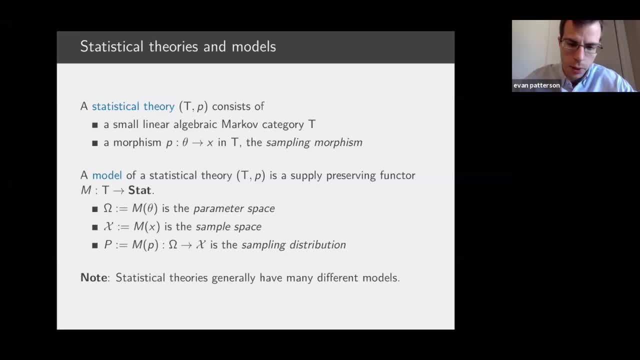 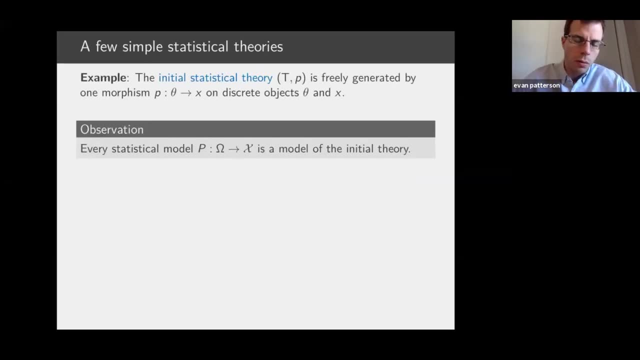 other. So one way that they might be related to each other is that they actually share a particular theory. Okay, so the simplest of all. well, the second simplest statistical theory is the initial theory, and it's just the theory that's really generated by a single. 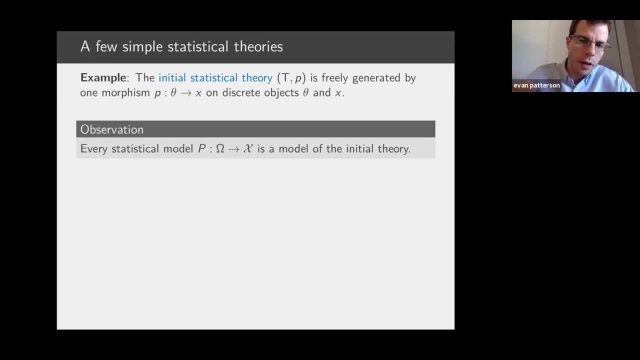 morphism on objects theta and x that have no additional structure. Okay, and then you can observe that, well, any statistical model in the classical sense is a model of this theory. So I just point this out, to say that you don't one doesn't one doesn't lose anything by adopting 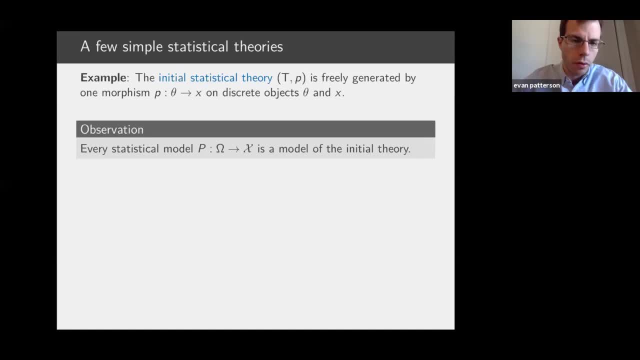 this. You can always take the sort of the trivial theory, but of course it's more interesting to put more things into your theory and then that more constrains the class of models. So another somewhat constrained but still quite general theory would be, say, the theory of NIID samples. 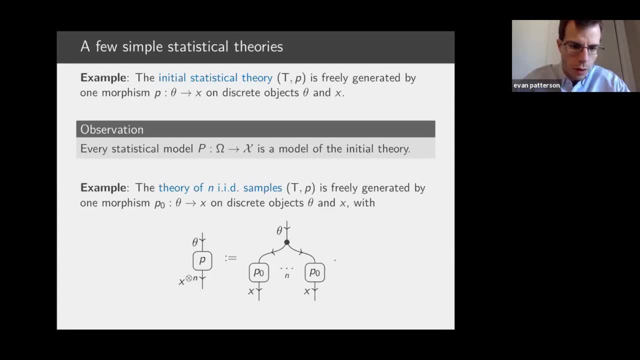 which just says that you start with again this generator, which we'll call p-naught, and then we define the sampling morphism to share that parameter, theta, and then have n independent copies of the data coming from this generator p-naught. So this: 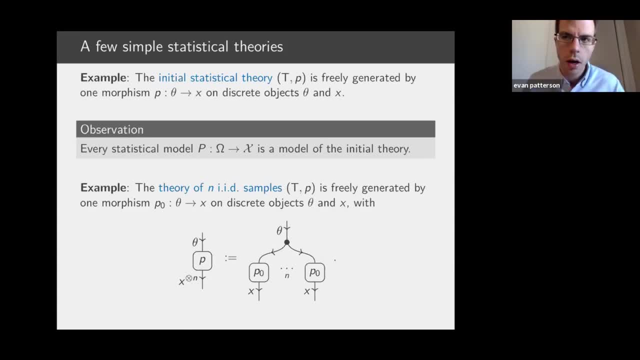 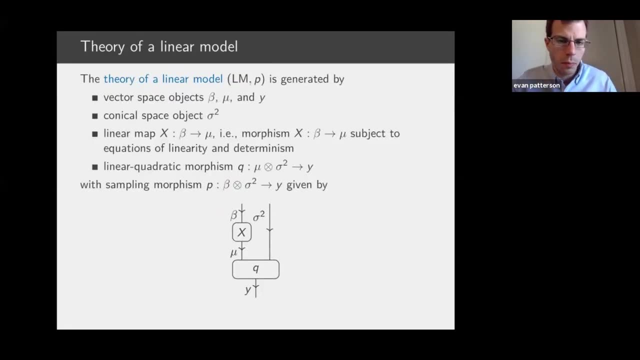 in other words, is the theory that describes any sampling distribution, which is an IID sample of n things. Okay, so more interesting theory. So this is making precise the example that we saw at the beginning. There is a theory of a linear model, So it'll be. 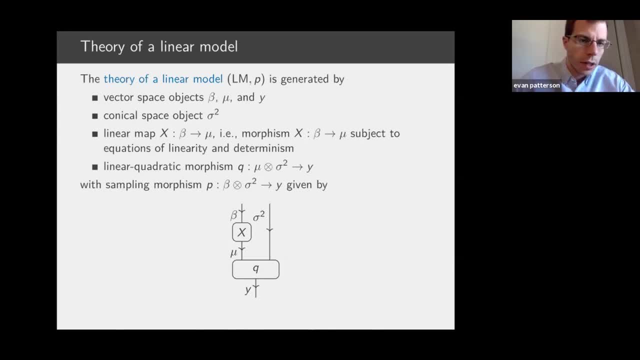 so the underlying category of it will be generated by some vector space objects: beta, mu and y conical space object, sigma squared representing the variance, a linear map which is going to represent the design, and then a linear quadratic morphism. 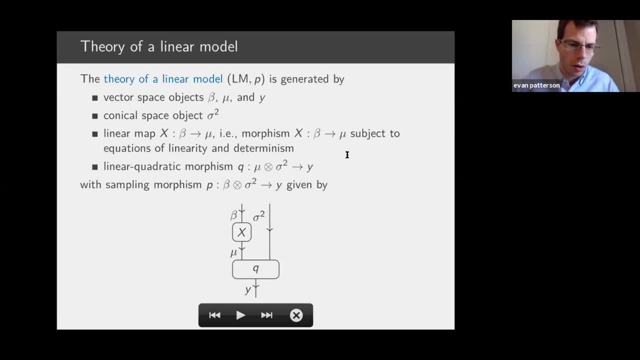 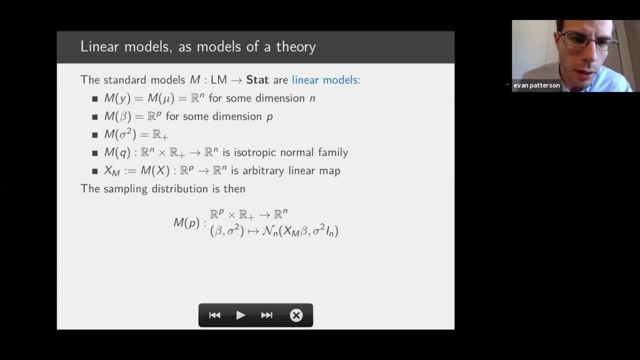 which represents the random part of the model, and then the sampling morphism is given by pre-composing the random part with the design matrix. Okay, and then. so to make clear how this idea of a model works here. so how do we get back the 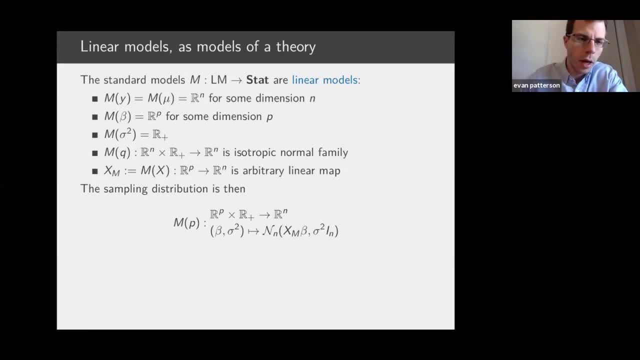 regular old linear models. Well, we assign y and mu to be Rn for some n, and the beta becomes Rp for some dimension p's, We'll just assign the sigma squared to be the non-negative reals. we'll take this random component to be the isotropic normal family and then finally, 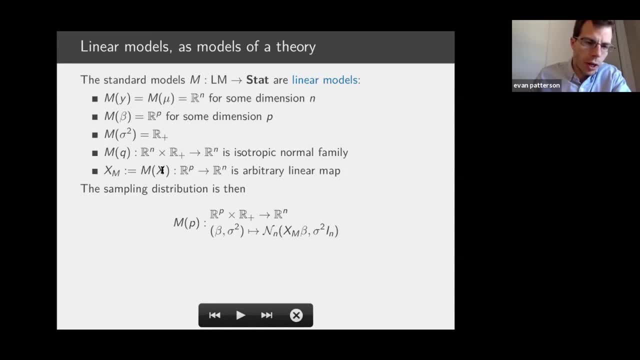 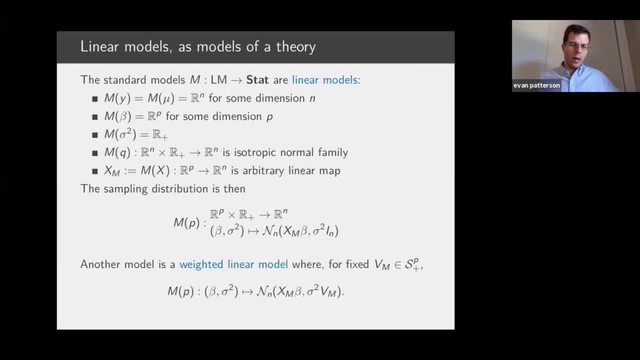 that there are, for example, some other models. So we've seen that these linear quadratic morphisms in general can have other models. So another model of this theory would be what's sometimes called a weighted linear model, where instead of having a spherical covariance, we instead 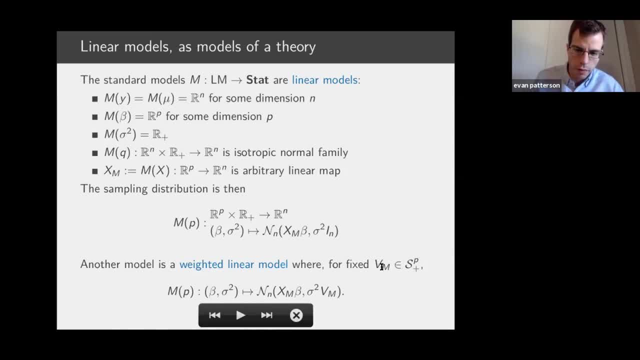 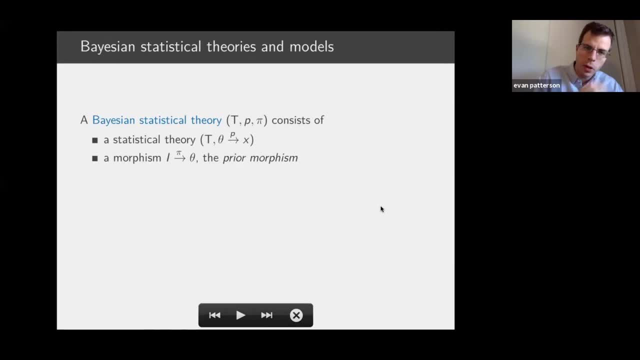 have it weighted by some other, by some generic fixed matrix v. Okay, and if you want to, you can add sort of the apparatus of Bayesian statistics to this pretty easily. So you could say that a Bayesian statistical theory consists of a statistical theory plus another morphism. 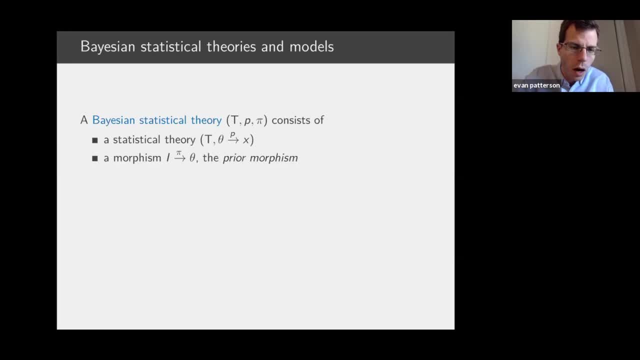 from the monodal unit into theta, which represents the prior and then a model of that. We're going to recover something which is essentially like a normal, the standard notion of a Bayesian statistical model. So it's a functor just like before, and then one gets sampling distribution, like before. 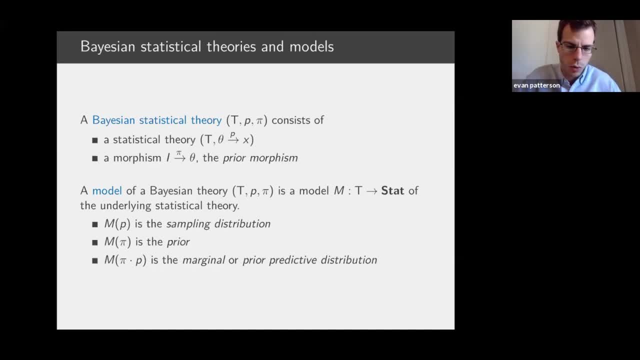 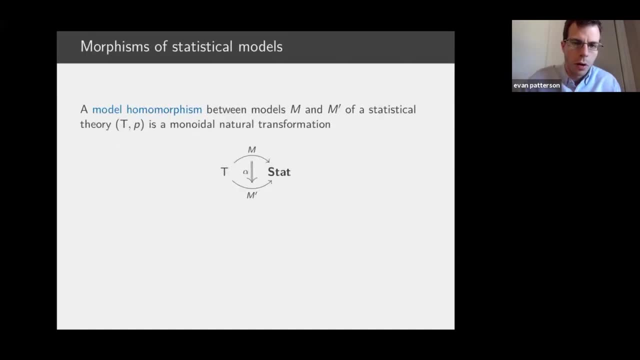 but now you have a prior distribution and then, by composing those, you also have what's sometimes called the marginal or prior predictive distribution. So one nice thing about this formalism is that, having set up this abstract stuff, one gets for free essentially the notion. 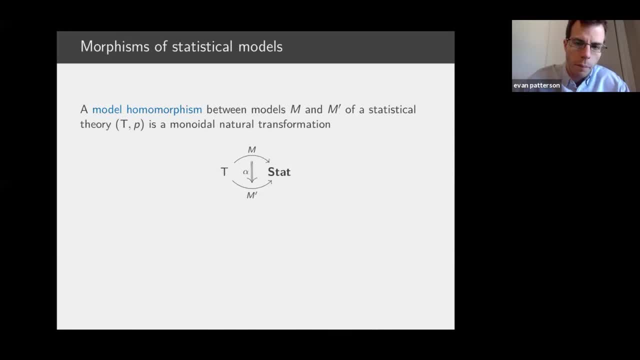 of a homomorphism between statistical models, which is not something that's often considered in statistics, So namely a homomorphism between two models which we would call are just functors is a monoidal, natural transformation between them, And one important thing to know is that 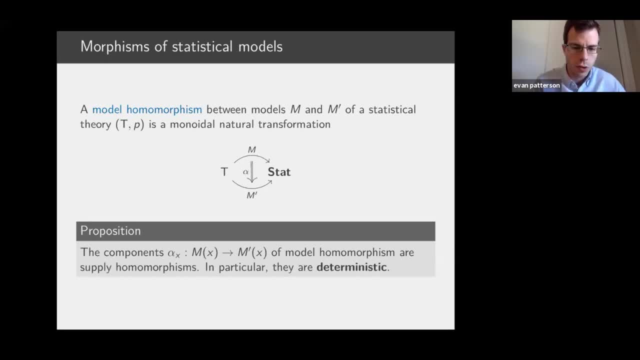 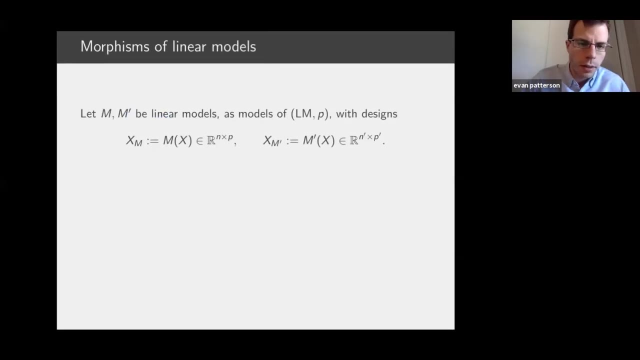 you can check that the components of these natural transformations have to be supply homomorphisms. So, in particular, that means that they have to be deterministic, which usually makes sense. So, for example, let's look at what the morphisms of the linear model are. So if I have two, 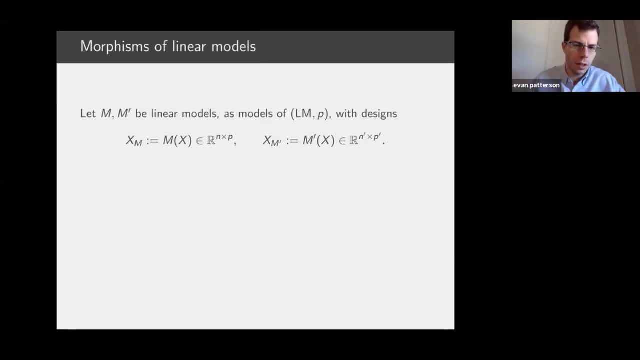 models m and m prime, which are both linear models, that is to say they're still kind of the standard models of the theory of a linear model, and then the corresponding design matrices are xm and xm prime. then you can check that a model homomorphism is uniquely determined by only two of its components. 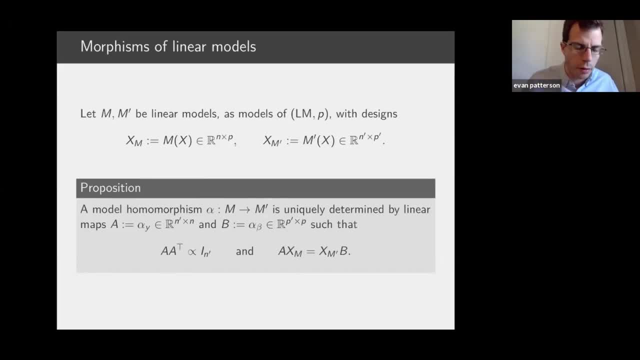 namely there's a linear transformation a of the sample space and another linear transformation b of the parameters, and they need to satisfy two properties: some or aako ré of, so that went to be NPC material, and theially, the transformation of the samples needs to be what sometimes called like like proportional to a semi-orthogonal. 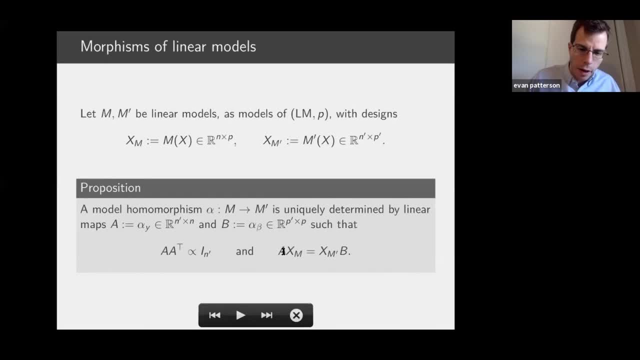 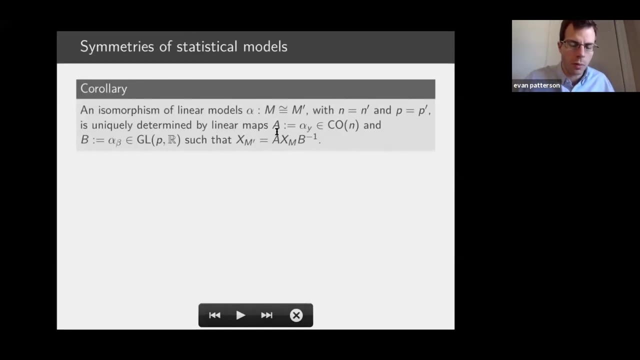 matrix or something like that. Basically, this is what's needed to preserve the spherical covariance structure, and then the two design matrices have to be intertwined. this gives a notion of isomorphism of linear models. So that only happens according to this setup when they have equal dimensions, if that makes sense. And then in that case, 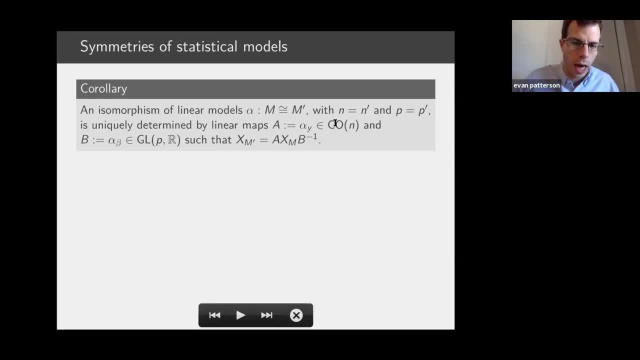 an isomorphism is uniquely determined by a linear map A, which can now be described as a conformal orthogonal matrix, as well as an invertible matrix B, which makes the design of M prime equivalent as a matrix to the design of M. That's fairly intuitive. So one thing I. 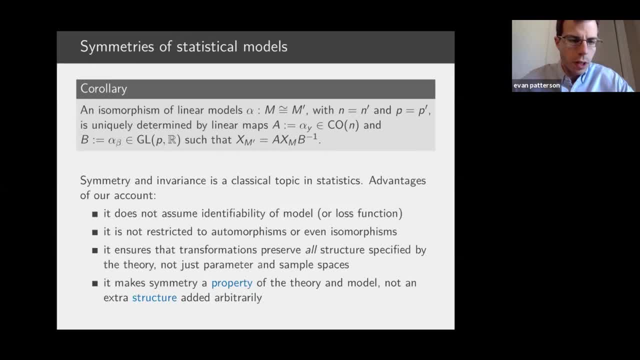 just want to point out about this. symmetry, sometimes called like invariance in this setting, is a classic topic in statistics. Books have been written about it, But I think there's a number of advantages to this account of symmetry over the classic one, which I'd like to try to. 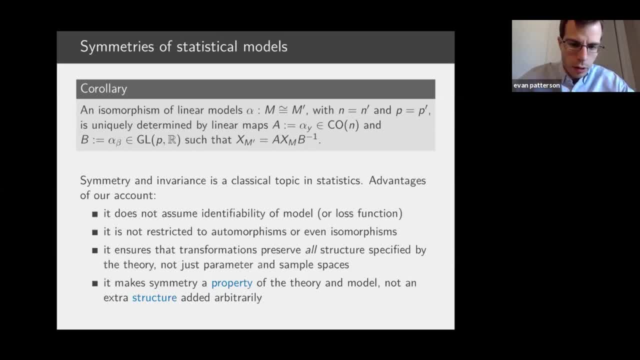 argue for One is that, and essentially, all of these advantages stem from the fact that we have available the concept of a natural transformation, So we don't end up having to assume things like the model being identifiable. I won't get into why that has to happen in the classical setup. 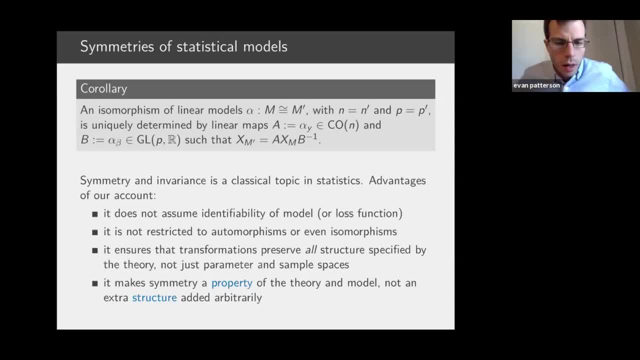 but it usually is assumed. More importantly, it's not restricted to automorphisms or even isomorphisms. So the notion of of morphism is applied to just regular homomorphisms And because we have the notion of a theory in place, 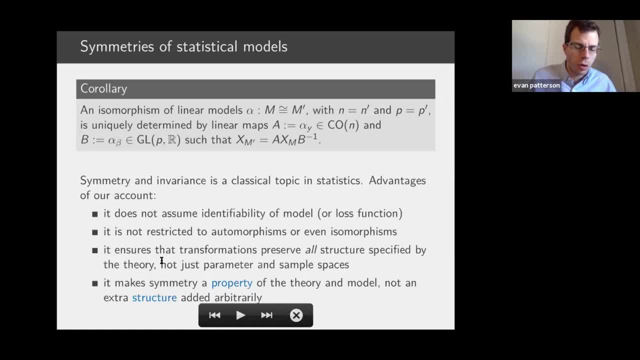 the morphisms, in this sense, have to preserve all the structure specified by the theory, Whereas in the classical setup you would just have transformations of the parameter and sample spaces, and then common sense is relied upon to ensure that you're not doing something which 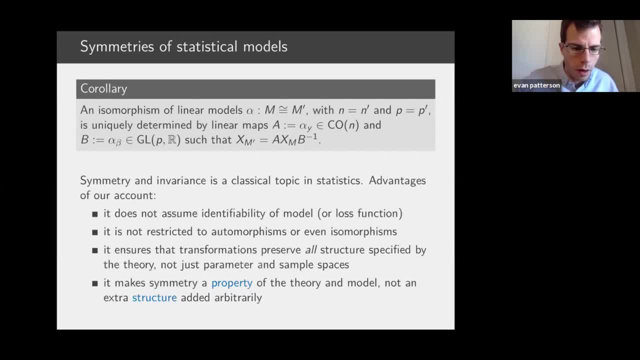 doesn't make sense with the other parts of your model. And then, perhaps most importantly, it makes symmetry a property of the theory in the model. So it's not something that you add on after the fact by applying common sense sort of ideas. It actually 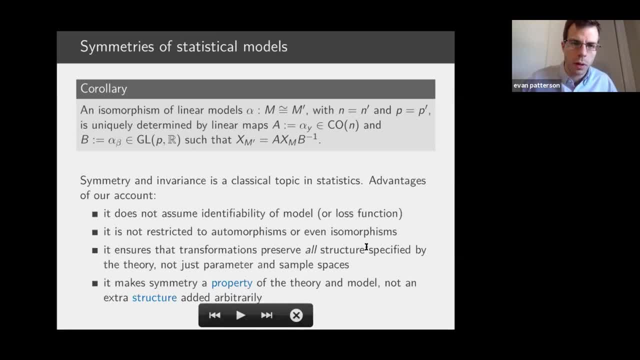 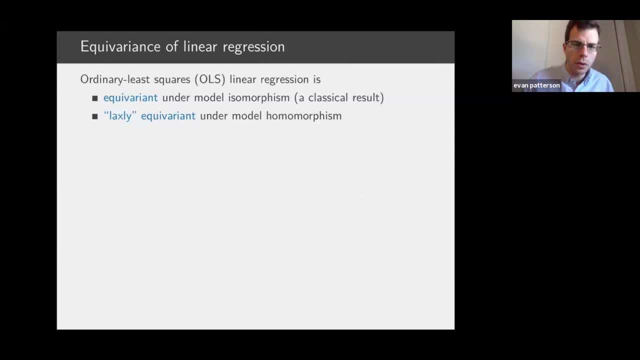 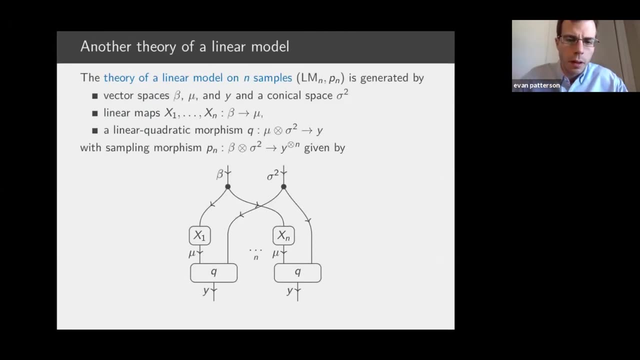 is a property of the theory and model once you've formalized it in this way. So anyway, so let me see, I'm going to skip this discussion of equivariance. So let's look at some, let's look at some additional theories. So the first thing to 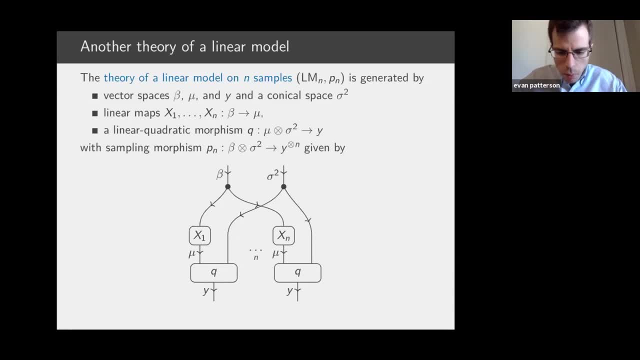 point out is just like models are just like a single theory- sorry, just like a single theory doesn't necessarily generally has many different models- a single model in the classical sense might have a number of different theories that describe it well. So another theory. 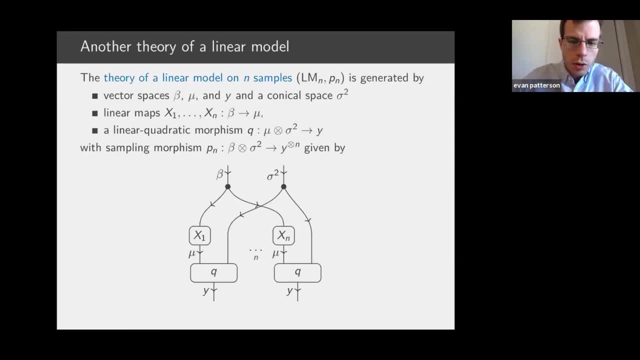 of the linear model is going to in this case, it's going to make the number of observations explicit in the theory. So here we're going to generate the category by beta, mu y and sigma squared, like before. Instead of having a single linear map, we'll have n of them. We'll have a. 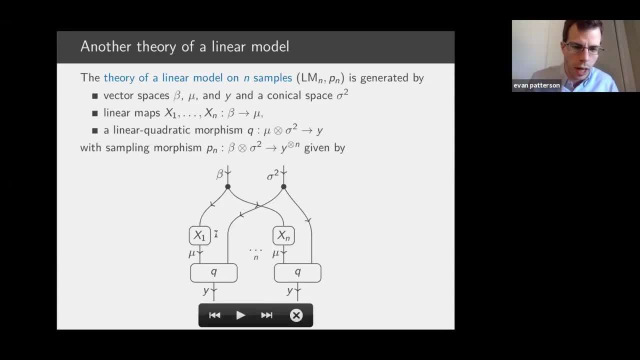 linear quadratic morphism, as before In the sampling morphism we'll have this structure. So we're going to have basically n, n copies And then of the of the parameters. we're going to hit it with the different parts of the design and then apply that to the, the, the random component, And so if 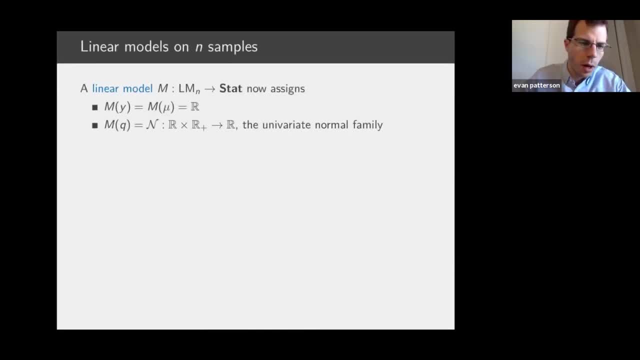 we want to get back from this, the standard linear model. the main thing that we're changing is that we're now assigning y and mu to be r instead of rn, And then likewise the. the random component is just the univariate model. 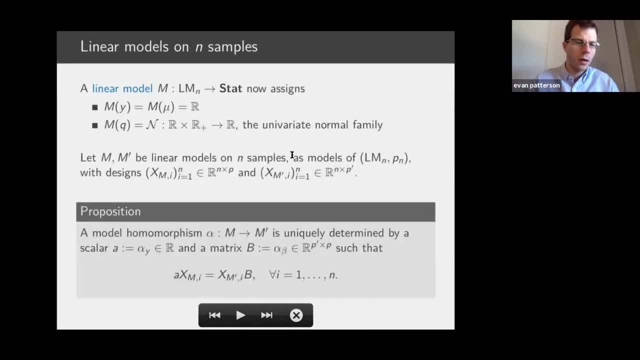 So if we do this, we get back the linear model. So one thing I want to point out is that, okay, so you, you get back the same class of models, But now actually the model homomorphisms change because you changed the theory right, So so now we get a stronger notion of model homomorphism. 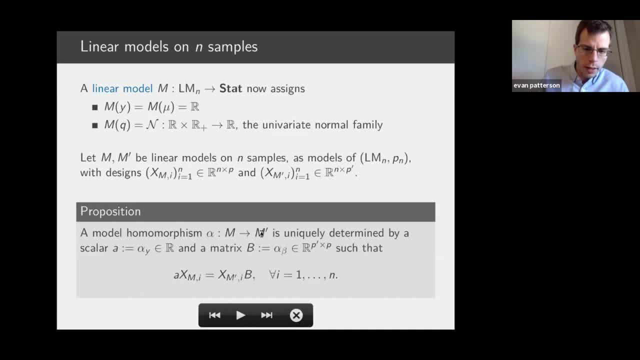 which is required where, where, the. instead of having a um, an arbitrary matrix transforming all of the observations, we just have a uniform scaling of the observation, of each observation, And then the design matrices have to be equivalent, but again in a stronger sense, they're basically equivalent across all the rows. 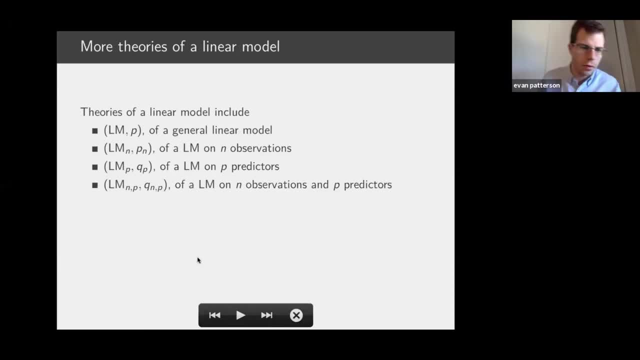 Okay, and- and you can come up with lots of other theories, right, You could, you can. in addition to making the number of observations explicit in the theory, you could make the number of predictors explicit. you could do both. 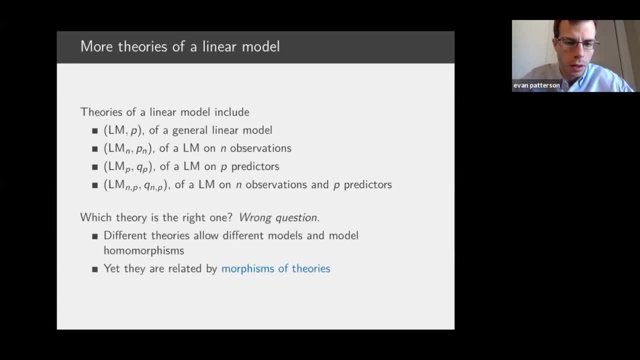 So you end up with a family of theories. So you might ask: which theory is the right one, Which one should I use? But that's not really the right question to ask, because, um different theories, um are more or less restrictive about their models and they determine different model. 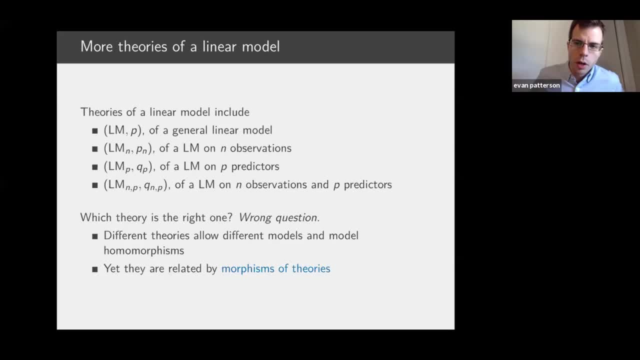 homomorphisms. So it depends, perhaps, on which structure you're um most wanting to insist on, But the important point is that the theories are related by um morphisms, So that if someone picks one and another person picks another, there's a way of saying that they're related to. 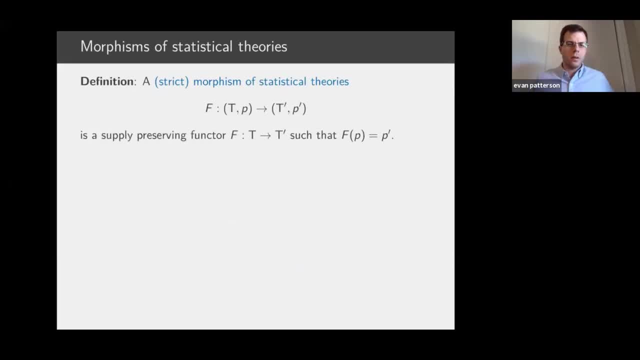 each other. Okay, so this brings us to the notion of morphism: statistical theories, Okay. so, um, if theories are, uh, a certain kind of category together with the distinguished morphism, then the most obvious notion of a morphism of theories, 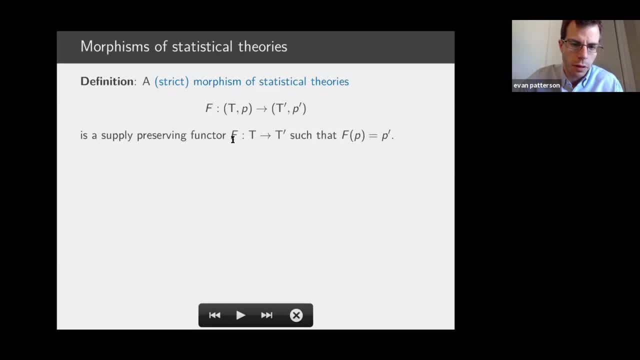 would be a functor, So in this case a supply-preserving functor between the categories, and then we'll ask that the for now, we'll ask that the um sampling morphisms be strictly preserved. Okay, and according to a uh, by now fairly familiar paradigm, this: 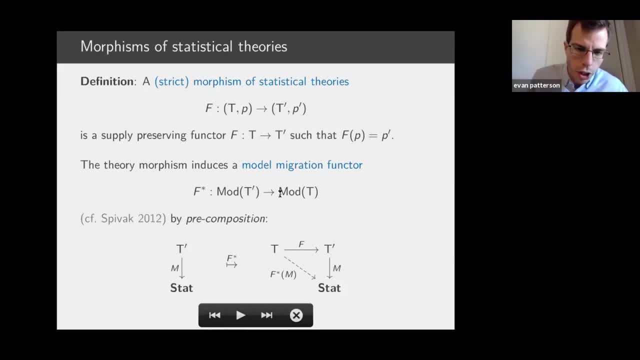 morphisms and theories induce um migration functors between the categories of models of those theories. So, and the simplest, the main way this happens is that if I have a model of t prime, then I can pre-compose that with a theory morphism from t to t prime to get a model uh of t. 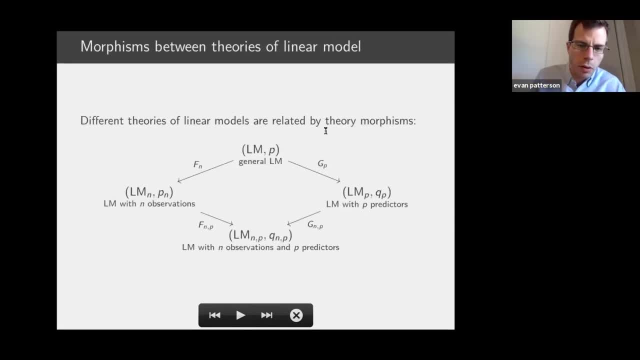 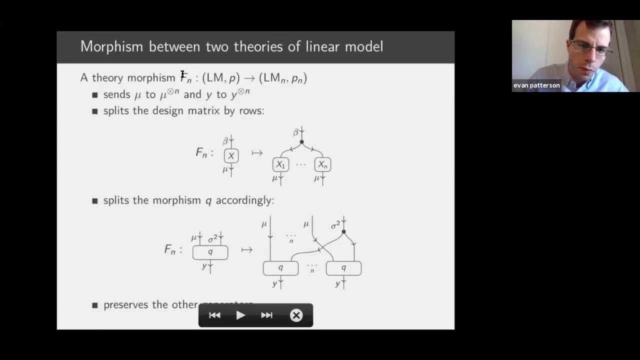 Okay, and so going back to our family of theories of the linear model, these are really um related by theory morphisms, And so let's see what one of those looks like. So for the two versions of the theory that we looked at, 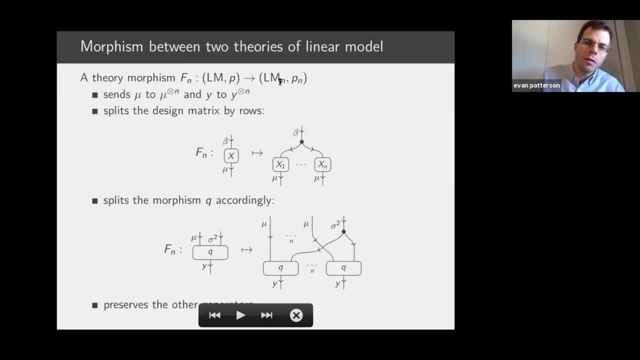 so the original one and then this one with the number of observations made explicit. well, to make that mapping, we can send mu in the first one to the infold product of mu in the second one. likewise for y. And so what does this correspond to doing? 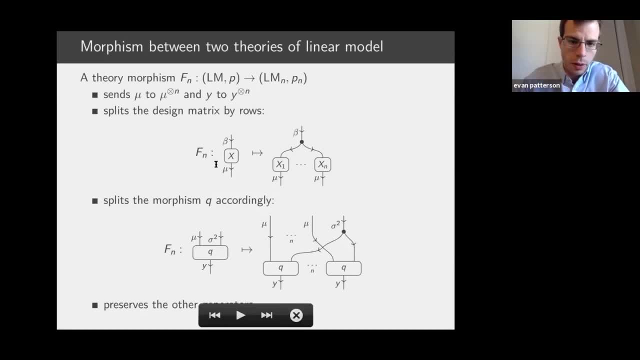 This is splitting the design matrix up by rows. okay, So that means that the design matrix in the first one should become this composite matrix in the second one, And then we have to split the random component similarly. So we do that here And then the other generators. we can leave them as is. 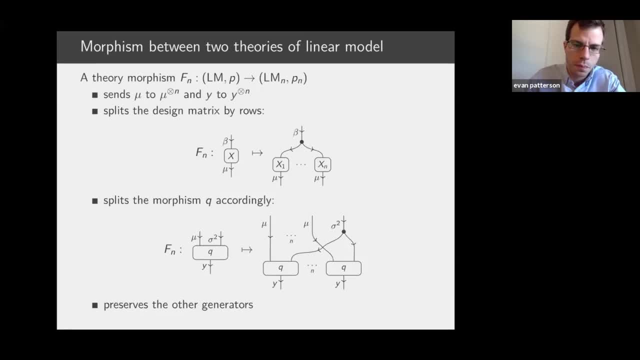 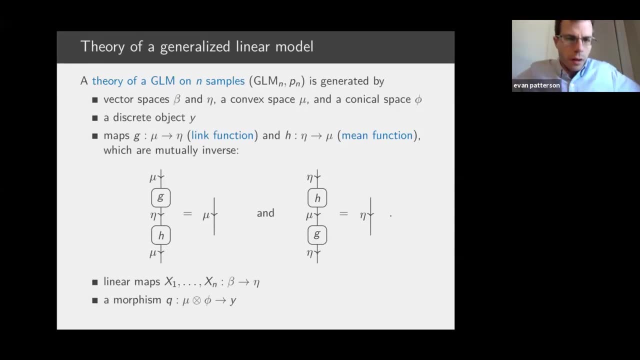 Okay so, and that defines a theory: morphism. So let's look at another example of a theory which is maybe a bit more involved than the linear model. So this is a theory of a generalized linear model. So if you don't know what that is, 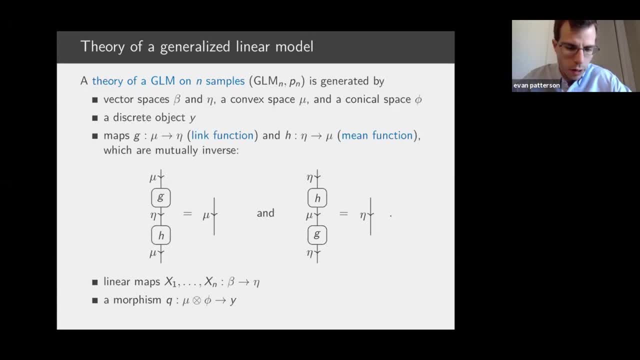 you can think that, if you're familiar with these things, that both linear regression and logistic regression are both particular kinds of generalized linear models. So, at any rate, the theory is generated by vector-space objects, beta and eta, convex-space, mu, conical-space, phi. 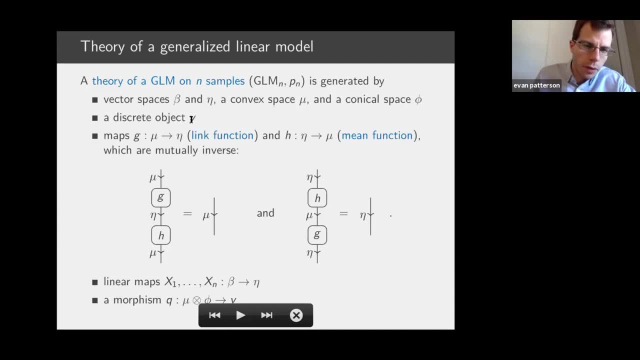 There's the discrete object y for the observations, So no structure assumed of that. And then there are these link functions which say how mu and eta are related to each other. So we ask that those be mutually inverse. there's again some linear components here to this model, which 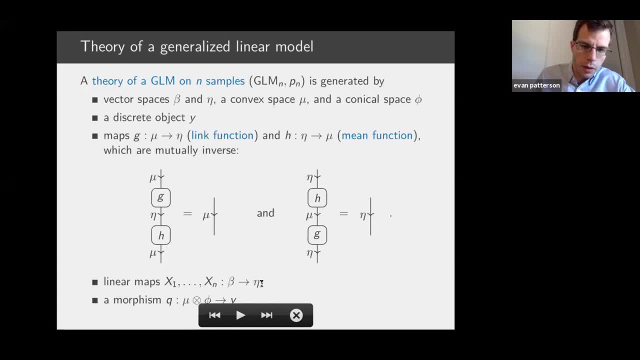 represent the parameters beta with these natural parameters, eta, and then there's a random component as well, and now we're no longer insisting that that random component really satisfy any properties. It can be arbitrary as far as the theory is concerned. So the sampling morphism then looks like this. So if 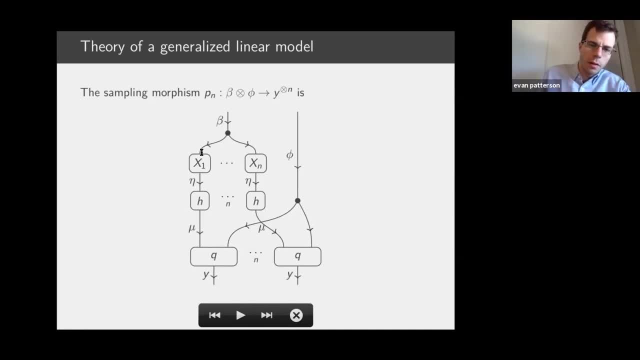 you've seen a GLM before, this will look familiar. If not, probably not. but in any case, what's happening here is we start with the parameters, we copy them, they go through the linear part of the model, then we're applying the same. 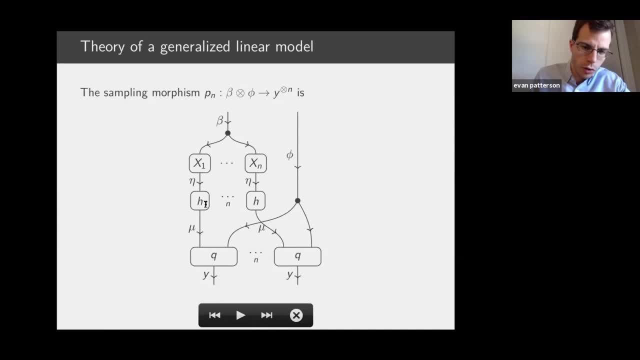 generally nonlinear transformation here. So this is what's taking us out of the realm of linear models. Generally this mean function is nonlinear and then those go to the random component of the model. okay, And so there's a stylized- you know fact that in statistics that well, a linear model. 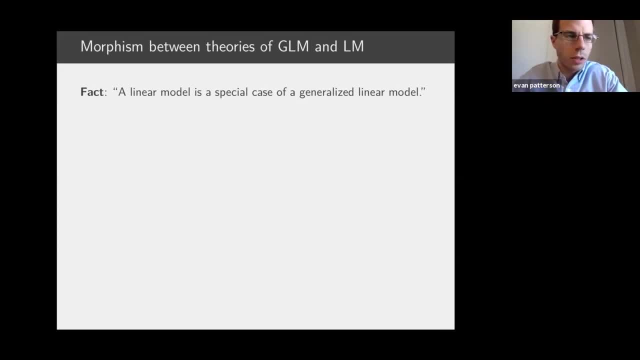 is a special case of a generalized linear model, and so the apparatus of theory morphisms allows this fact to be rendered in a very precise way. So, formally speaking, we can define a morphism from the theory of GLMs into that of linear models in this way. So we're basically going to collapse that. 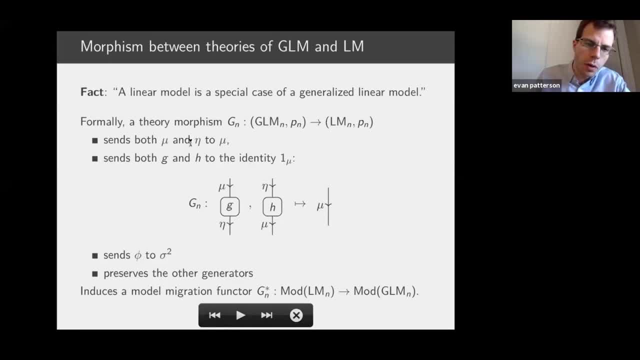 we're going to collapse the theory down, So it means we're going to send both mu and eta to mu. then we're going to collapse the mean and link functions both onto the identity. The dispersion parameter phi just becomes the variance parameter in the linear model and then we're going to leave the 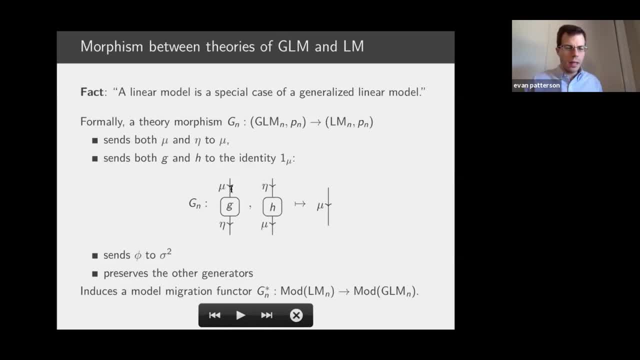 the other generators, as is. And this theorymorphism induces a model migration functor in the way that we've seen, And then if you unpack what this is doing, we'll see that you'll see that applying this functor to a linear model gives the corresponding normal GLM. So the GLM 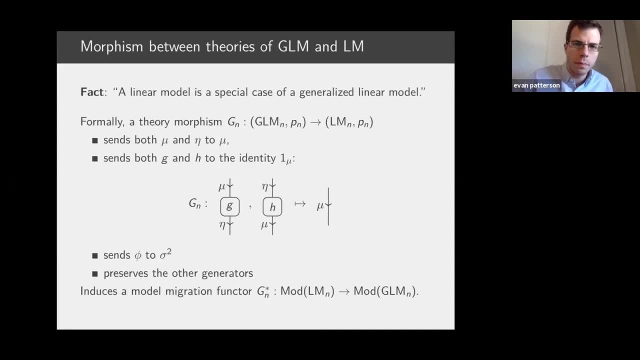 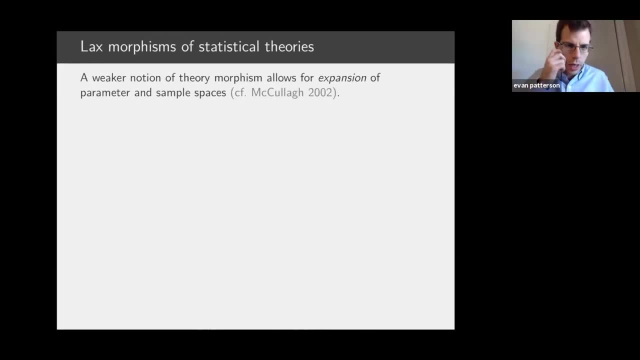 corresponding to the normal family. Okay, so I'll do this last part quickly, since we're running low on time. I'll just say that there's, in addition, a notion, a weaker notion- of theorymorphism, which allows the parameter and sample spaces basically to change. 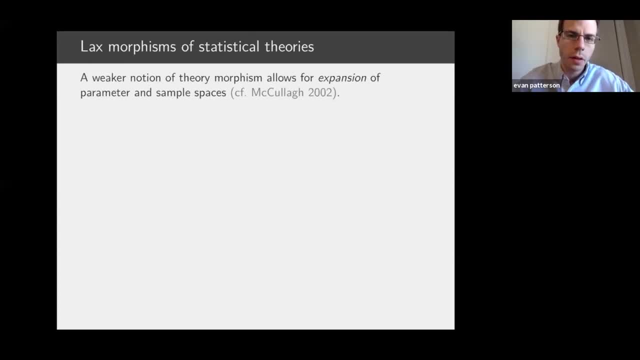 between the corresponding theories, And I think this notion is related to Peter Mercola's work on statistical models. At any rate, there's this lax, there's a notion of a lax morph in statistical models which has a functor just like the four. But then, instead of requiring 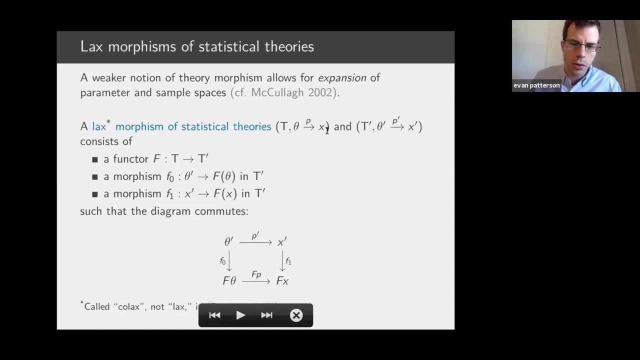 that the sampling morphisms be exactly preserved. we allow the domain, the sample space objects and the parameter space objects to go to different objects, But then they have to be these additional morphisms between them in t prime in such a way that this diagram commutes. So maybe an example will illustrate. 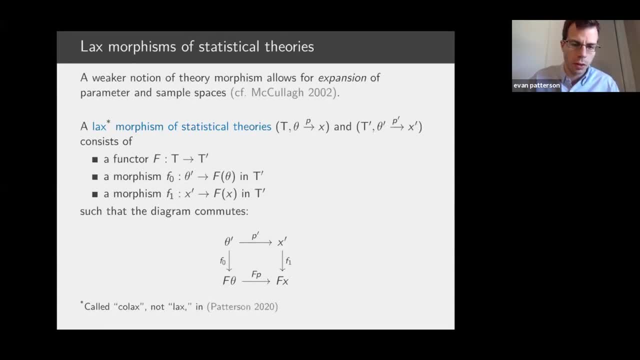 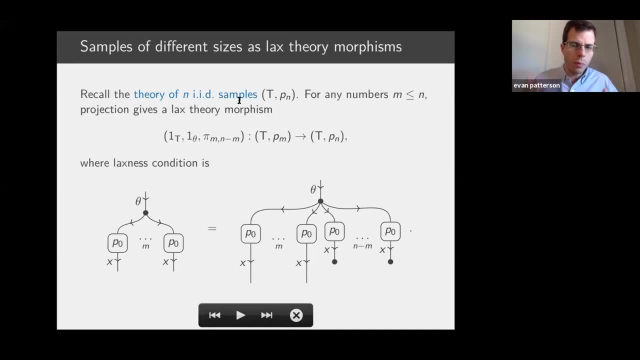 what the point of this, or a simple example will illustrate what the point of this definition is. So in the theory of IID samples, it seems, one might naturally want to think that there's some kind of inclusion, say between the theory of IID samples of some number into one of a bigger number, And that's the sort of 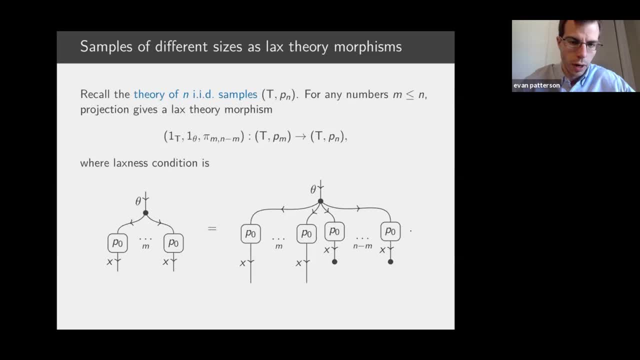 one of the sorts of things that this definition lets you express. So there's not a strict theorymorphism between these theories, but there is a lax one, And it works by basically discarding the last elements of the theory with more samples. Okay, so let me wrap up here. 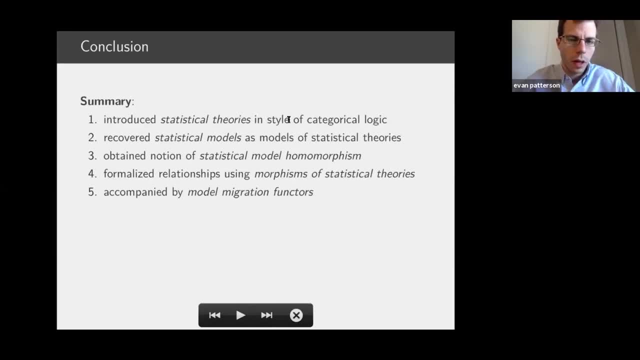 So what have we done? So in this work I've introduced the notion of a statistical theory, sort of modeled after the way these things go in categorical logic, And I've shown how the classical notion of a statistical model can be recovered as models in the logical sense of. 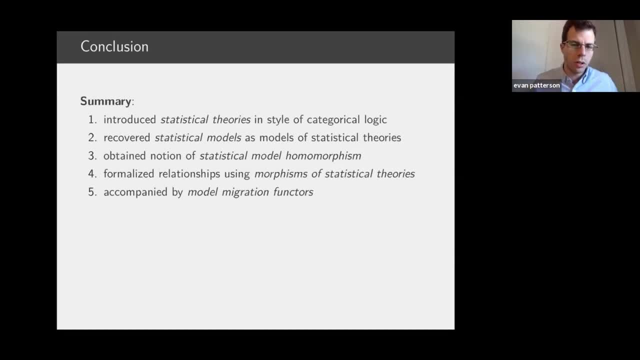 statistical theories. I've shown how this leads to a notion of morphisms between statistical models, And also how there are morphisms between statistical theories, which can be used to formalize relationships between different methods, And then, moreover, these morphisms and theories. 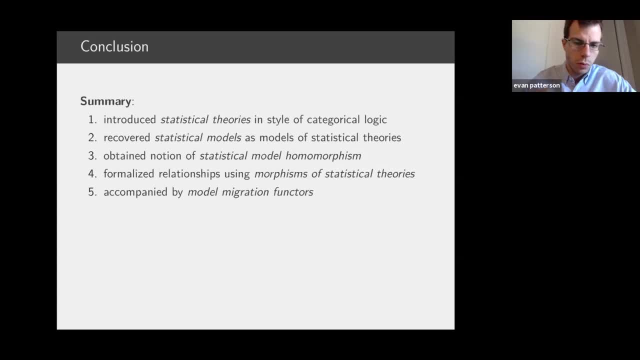 further, give you model migration functors between categories of models. Okay so, and where might one go from here? Well, I think there's lots of things one could do. So certainly, there's probably more work to be done on this, but I just want to give you some examples of things you could think about. 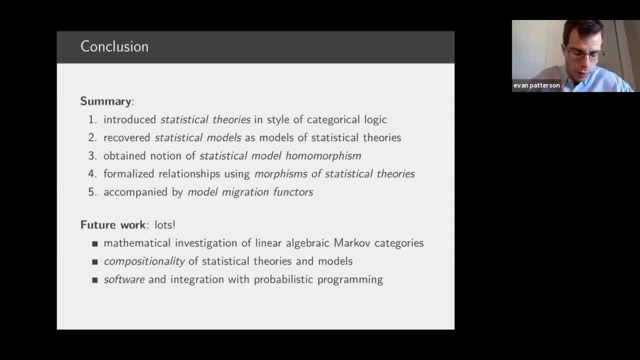 on studying Markov categories and linear algebraic Markov categories and things in that space. There are definitely people working on that. One thing that I didn't address in this work, which should be addressed, is the notion of compositionality of statistical theories and 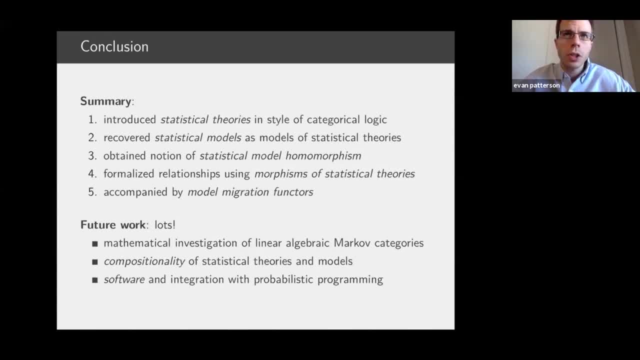 models. So, in other words, like you know, especially in certain kinds of Bayesian or hierarchical models, one thinks of them as being composed out of simpler ones, and that should be brought out and made formal. And then one thing that I'm certainly interested in: 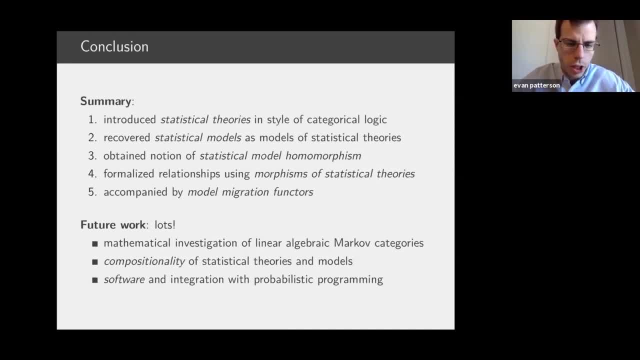 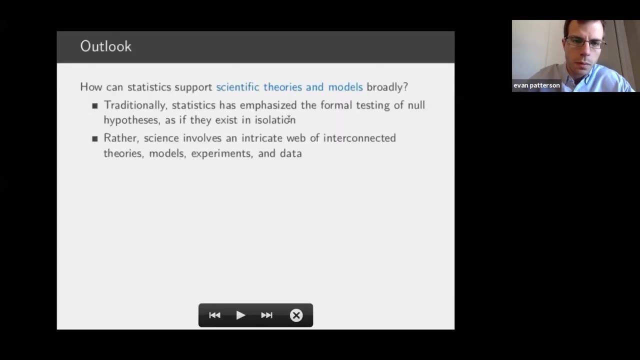 doing is trying to instantiate these mathematical ideas in software, for example by modeling statistical theories in code and perhaps integrating them with probabilistic programming languages or something of that nature. Okay, so here's the general sort of outlook that I'd like to leave you with. So one question that I think it's good to ask. 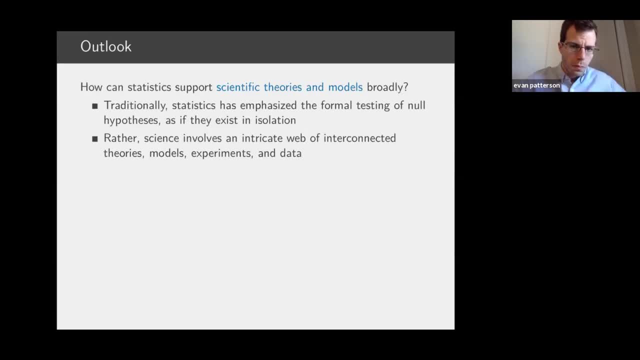 is what is really the role of statistics and scientific theorizing and modeling broadly? So traditionally, at least going back to the early 20th century, statistics has emphasized the formal testing of null hypotheses. And if one really takes that paradigm at face value, 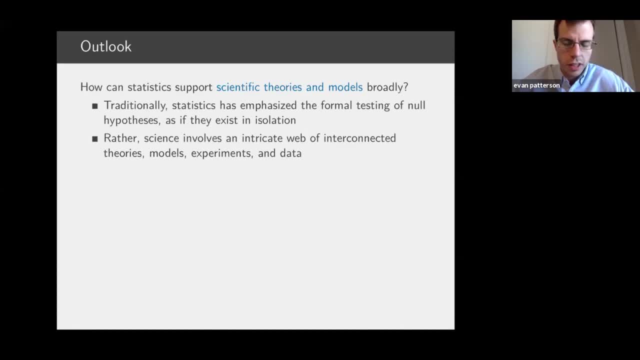 it almost appears as if these null hypotheses just sort of exist in isolation, and then every paper just puts forth a null hypothesis taken in a vacuum, When of course in reality the data is not a disconnected body of isolated null hypotheses. It is an intricate web of. 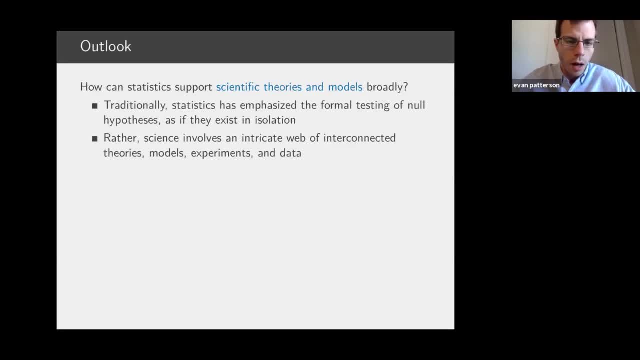 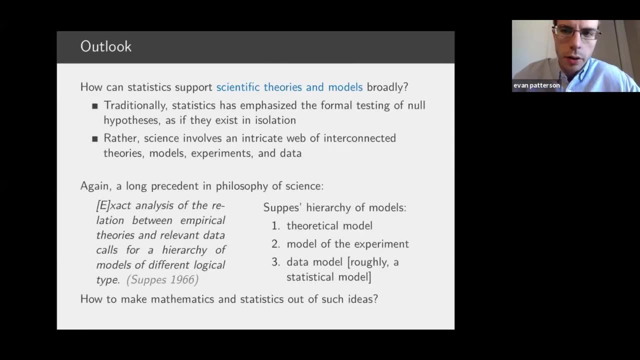 highly interconnected theories, models, experiments and data, And so it would be nice to try to model this in a more formal way too, And, as you would expect, this also certainly has a precedent in philosophy of science, not just with SUP. 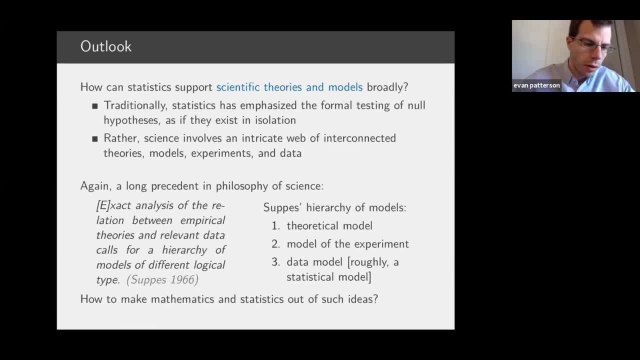 but since I quoted him earlier, I'll quote him again here. So here he is in a slightly later paper, in 66, saying: the exact analysis of the relation between empirical theories and relevant data calls for a hierarchy of models of different logical types. So he proposes a hierarchy of 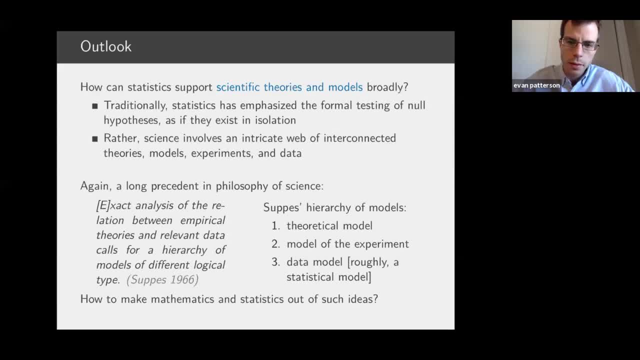 models to try to formalize this sort of the scientific experimentation and theorizing. His approach is just one approach. So I think a broad, broad question for people interested in categorical statistics to think about would be to how to really make more, make these ideas more systematic, So that I mean that's. 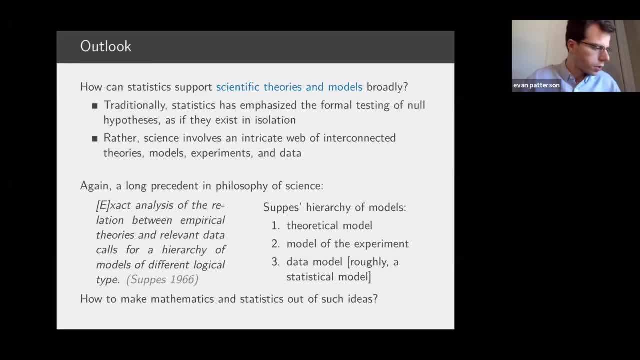 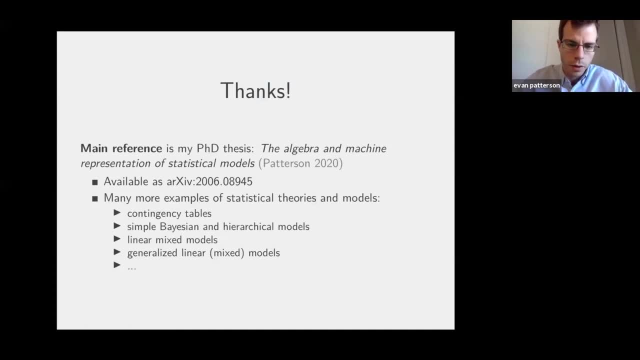 another general direction to think about. So I'll stop there. Thanks everyone for your time and attention. So if you're interested in this, the main reference is my PhD thesis, which is: you can find on my website my PhD thesis, which is: you can find on my website my PhD thesis, which is: you can find: 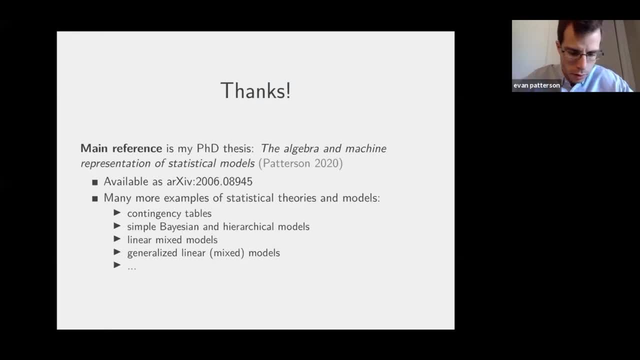 on my website my PhD thesis, which is you can find on on the archive, And one thing that's in there that I couldn't really do justice to. here is a really large set of examples covering things like contingency tables, some basic Bayesian models and hierarchical models, linear mixed. 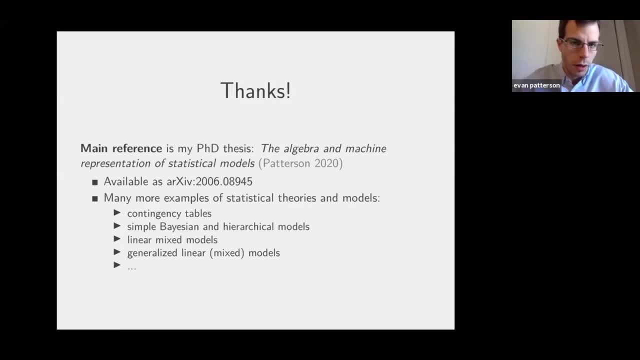 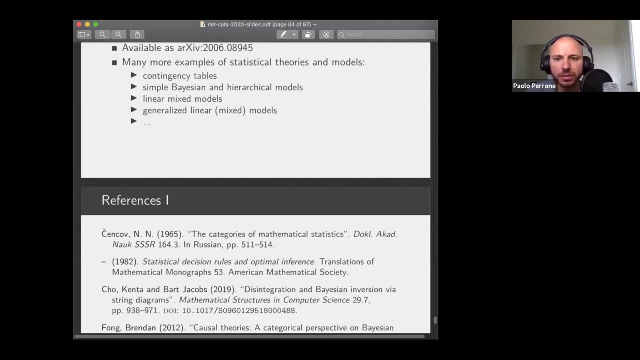 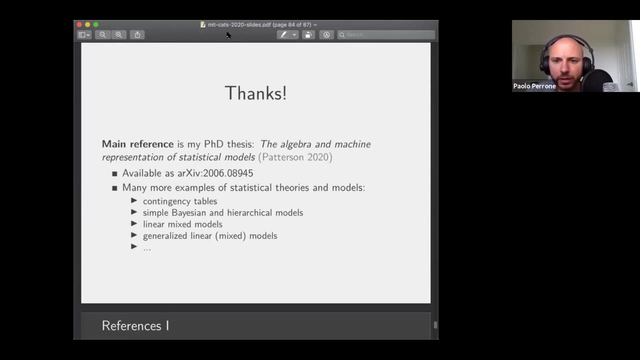 models, generalizations of those and other things. So that's what you'll find there, among other things. So again, thanks, And I'll stop there and take any questions. Thanks for your talk. Thanks a lot, actually Very interesting. All right, So I think you should now all be able to unmute yourself if you want. So Arthur had a question, if I remember correctly. 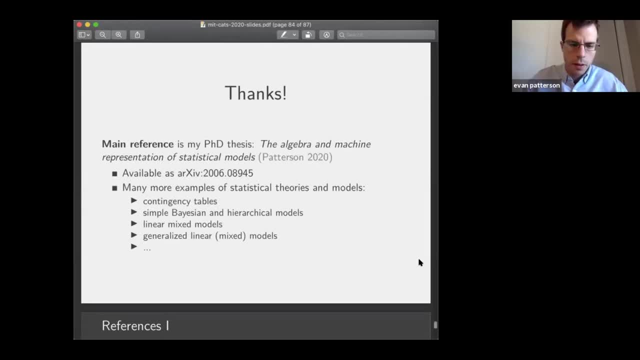 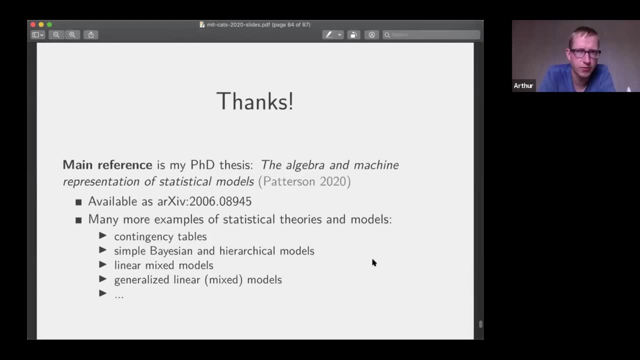 Yes, Yes, but I'm pretty sure it's been answered. So my initial question was: what makes a model linear, And is it the fact that the parameter space is a vector space? But correct me if I'm right or wrong. but 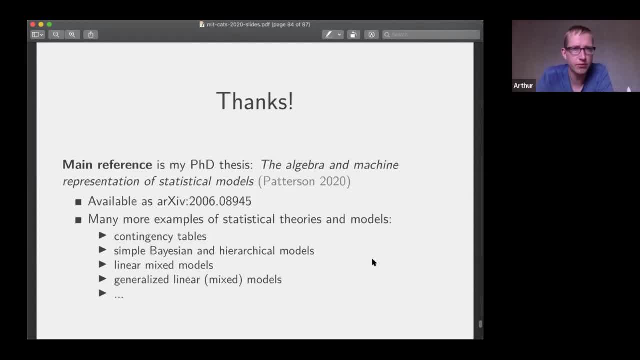 it's that plus more the morphisms in your category, or linear transformations. essentially, Exactly, Yeah. So it's not enough that the parameters live in a linear space. They need to be basically related to the mean of the sample vector in a linear way. Yeah, 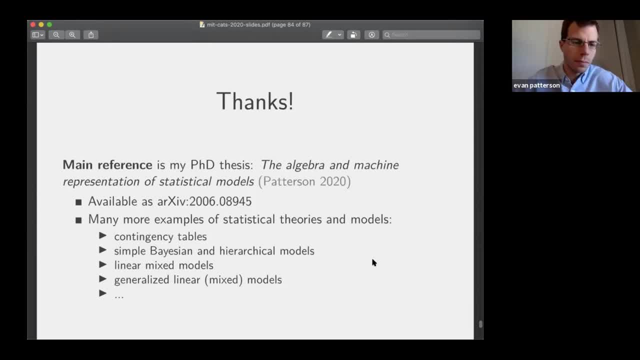 That's right, Thank you. So I had another question, if I may Sure. So there's been some work in the past 15, 20 years generalizing Tarsky and semantics to context involving metric structures, some model theorists, Ward Henson and some of those people. 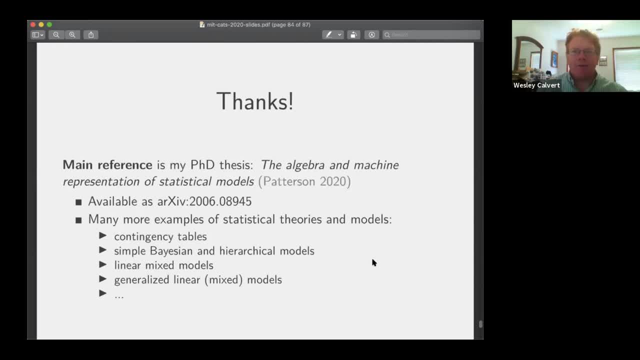 continuous first order logic. I know that there is fairly well established crosswalk between what things mean in classical first order logic and what things mean in categorical logic logic. They have theories of random variables in this stuff. I wondered if there's been any work on figuring out what the crosswalk is here. 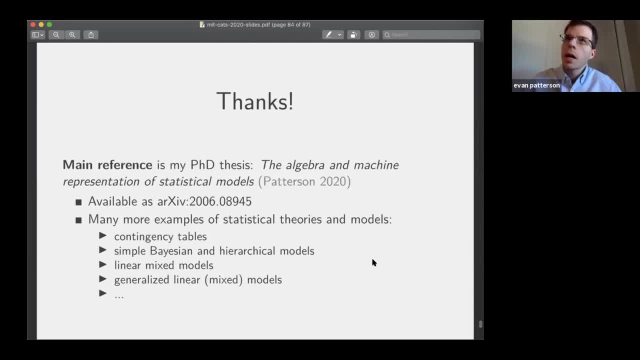 Yeah, um, that's not an area I know really well. I mean, I know that I'm not sure if this is exactly what you're referring to. I do know that people have tried to build like first order probability logics and stuff. We're trying to combine the probability theory. 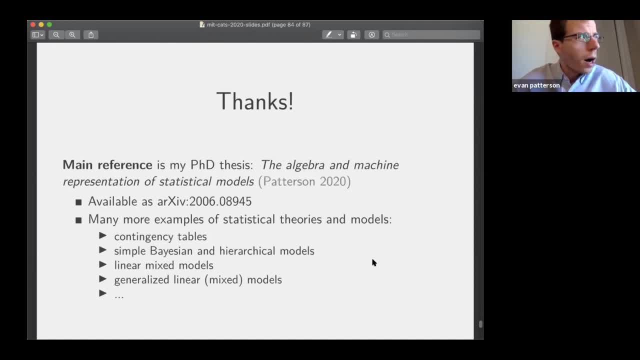 with first order logic, things like that. Um, so I don't know that I have a good answer to this question. I mean, I think that, from what I understand, a lot of sort of the existing work on probability and logic is. excuse me. 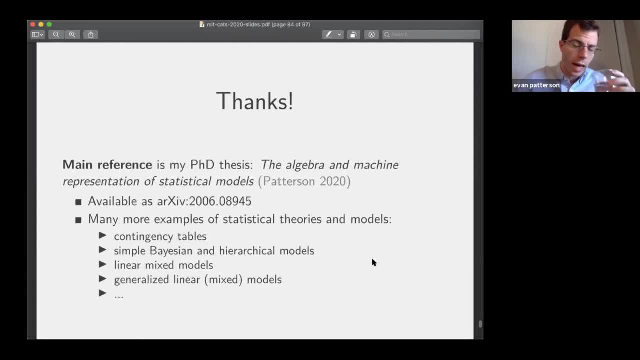 More focused on the probability than, like, the statistical aspects of it. So in this project I've really been focused on understanding statistical models. But yeah, if you have any pointers to relevant things or I'd be happy to look at it more offline and see if. 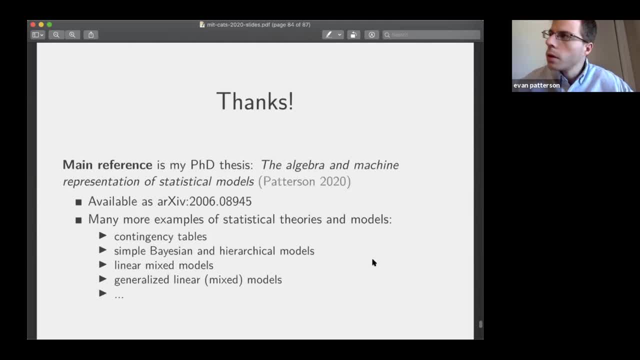 I can give a better answer to that. Thank you, Yeah, I had a question. Yeah, So the way I'm thinking about it, all these different wires are supplying different things. So for each wire, I can decorate it, I can split it or I can combine it or I can do. 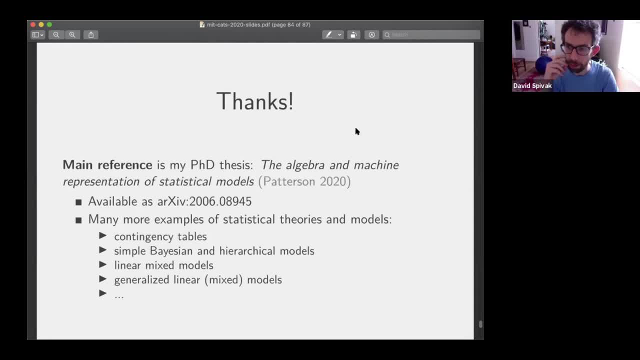 all sorts of different things With a wire labeled A. if it supplies prop P, then I can do anything P says I can do, But I didn't see so many uses of that. I remember seeing a little C where you were multiplying. 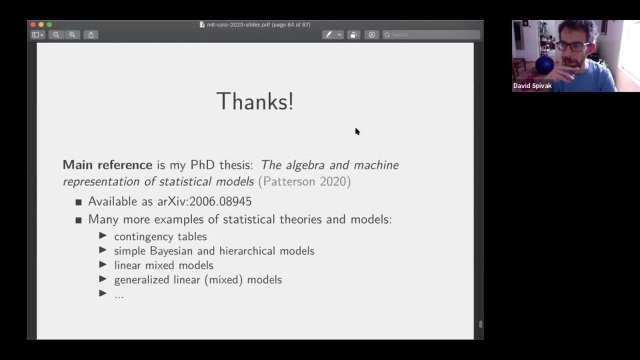 by a constant at some point And I definitely saw you splitting wires. I didn't see that. Yeah, I think you're splitting wires a lot, Yeah, But I didn't see that much of the other ones And I'm wondering if they're implicit. 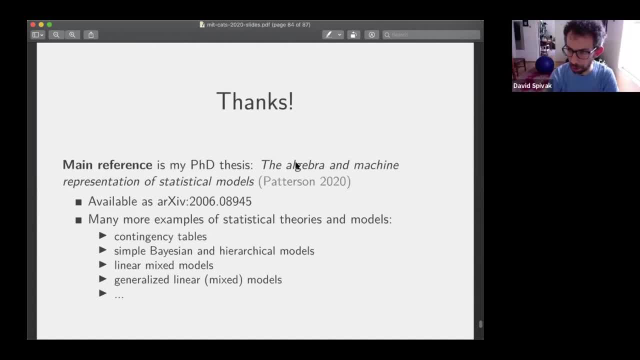 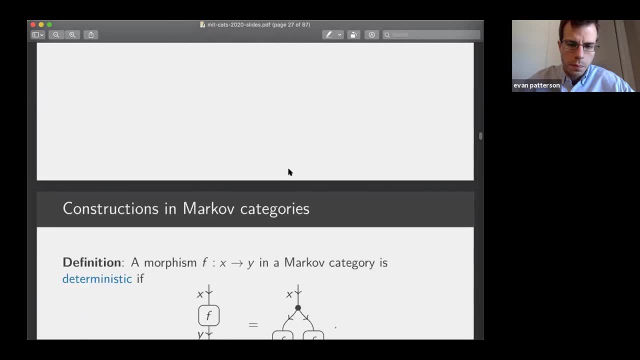 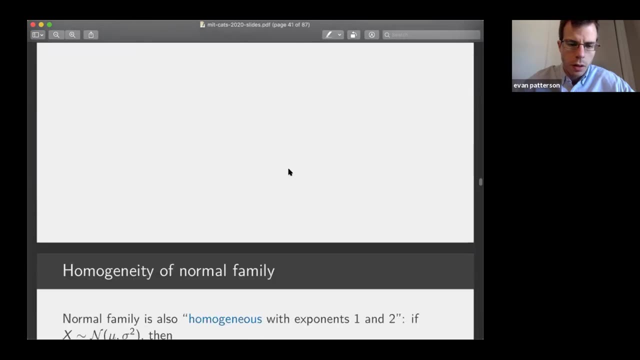 somehow like the way that a statistician would use these things. they would start to use those supplies, or Yeah, Let's see. So, let's see, We have Right. So here we're using, There's a time C, right? 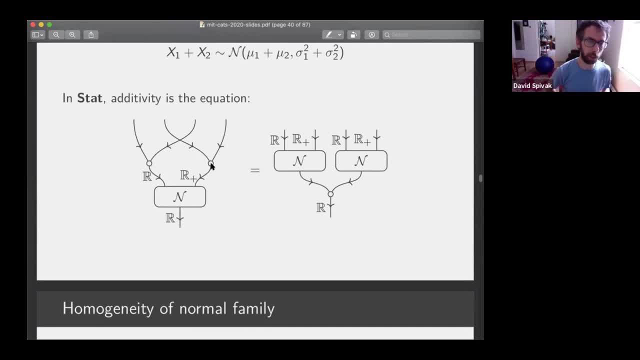 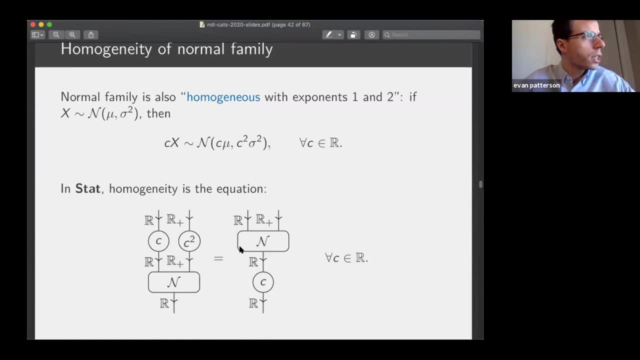 Right. So here's the plus. Oh, there's plus. Yeah, Okay, Merging, Yeah, Yeah. So you know, there's some things like: there's multiplication by C, there's copying- Those are honestly the biggest things- Adding stuff, scalar multiplication, that stuff There's. 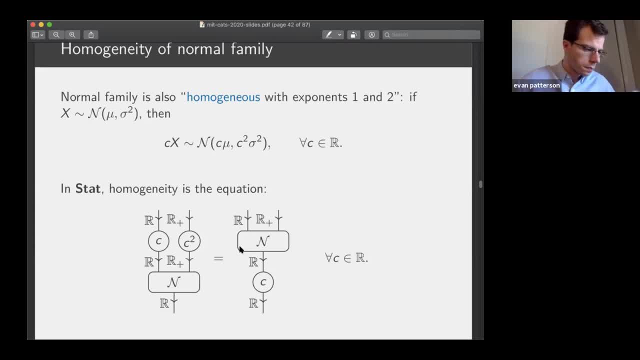 In the paper- Sorry, In my thesis there's examples of models of discrete data, like contingency tables, where you use convex, You're using convex, The convex structure, So that's a C structure more so that's not in the talk, but so I can if you want to see some. 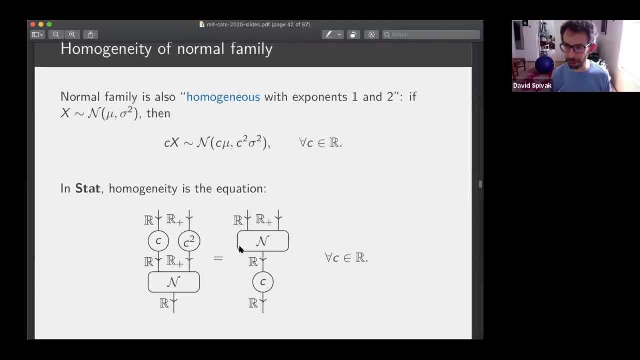 other examples where I think it's help. I think I just wasn't noticing when new you're using it. so thanks, yeah. well, it's just sort of very naturally creeps in there and you know right. think about it, right. yeah. yeah, that's lovely talk, thank. 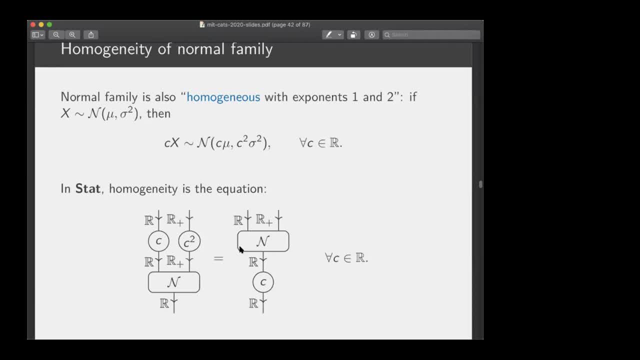 you very much for kind of connecting pieces. my question is about symmetry because, yeah, saying that symmetry is not an afterthought, it's actually built in, yep, and I was wondering whether- what do we know- that we actually want it all the time. I mean, I was thinking just more, you know, philosophically speaking, the 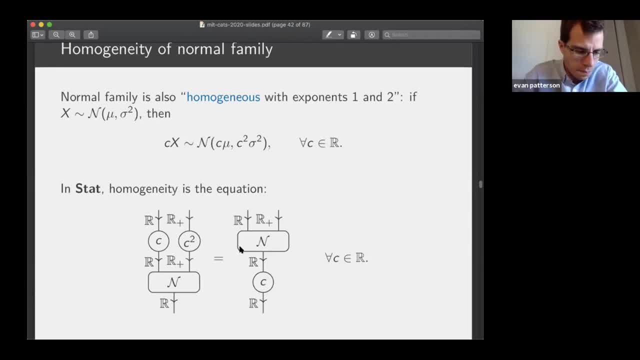 category theory. yeah, so there are, there are- sorry, excuse me, so there are different views, and statistics on how important symmetry is is a yeah, so some people have advocated that symmetry is actually a very useful principle for, like singling out classes of estimators that are at covariant under the relevant symmetry. 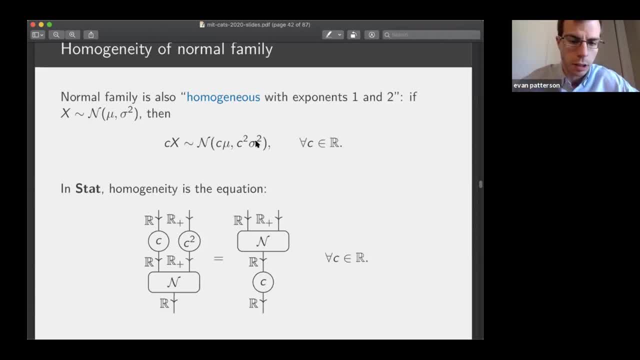 so I'm just wondering if you could give us a little bit more detail about that. yeah, so there are different views and statistics on how important symmetry is, so it was a way of constraining the space of possible estimators, in some cases even determining them uniquely. but some people have also said: we'll look. 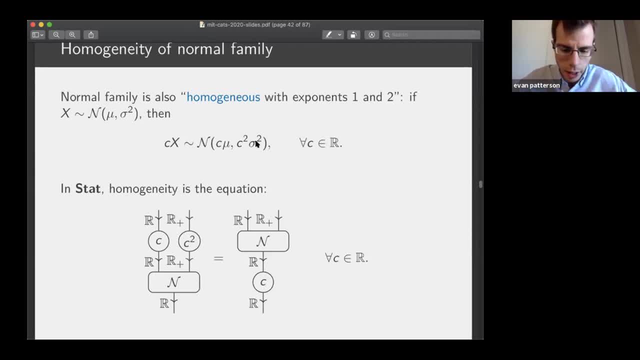 like. in practice, it appears that, like usually, you have prior information which would make, like, the geometric symmetries be less plausible, right? so, like you know, you're measuring something on a certain scale. you know, you're, you know it's not like you're gonna treat the whole real line symmetrically because some value. 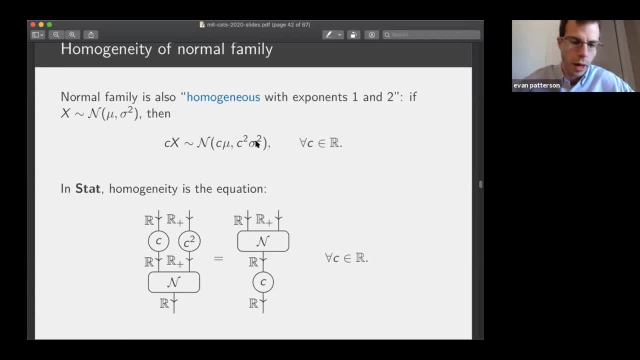 is like bigger than the size of the universe or something right, so like. you know so, but this is actually captured by the formalism. so like if you introduce like priors into the theory and in the model, like in the Bayesian sense, often what happens is the space of symmetries, unless the priors are set up in a 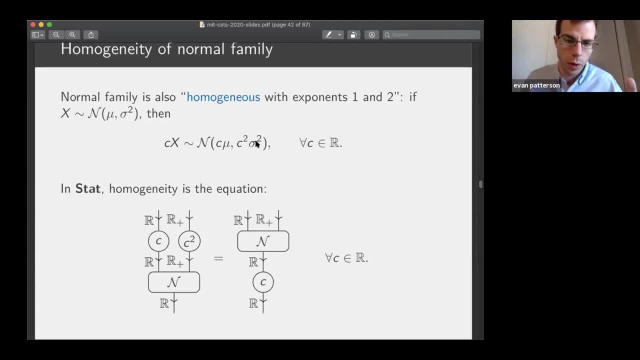 certain way that often actually will destroy the symmetries and you end up with very few of them. so so, um, just, yeah, let me point that out. yeah, okay, um, interesting, interesting. and another thing that I've seen passing by, so it's: I know nothing about the subject, so just you know, taking it with a grain of salt, but I've seen people 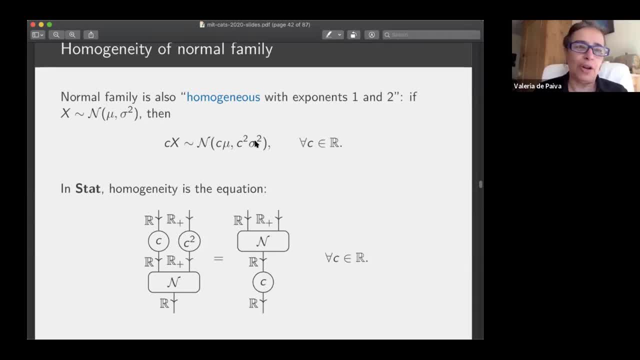 talking about orbits in in probabilistic logic and I was wondering if you have any ways of dealing with um orbits in the sense that that things that you know, like you have them in geometry, kind of, you apply transformations and you, you, you keep going until you come back to the same. 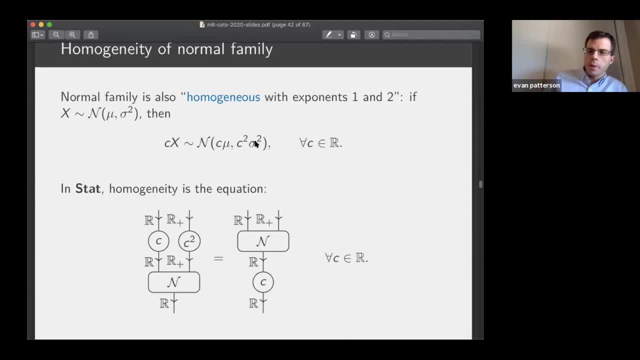 yeah, I haven't really thought about that. I'm not. I'm not sure. um, I'd be curious to know how they're they're using them in that setting. so, yeah, no, I have a paper, I can send it to you later, someone who's doing that. so I'm curious to know how they're using them in that setting. so 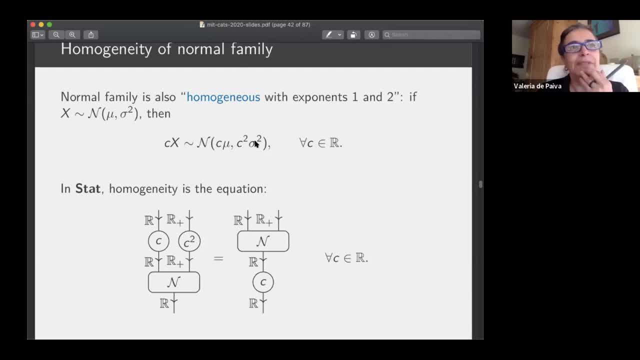 kind of stuff with kind of probabilistic logic in symmetry. so that's, that's why it can come in. the two questions come together. thank you, um, yeah, hey, very nice talk. so I'd also like to understand the role of the linear algebraic supplies a little better. yeah, so maybe as a sort of follow-up to David's question. 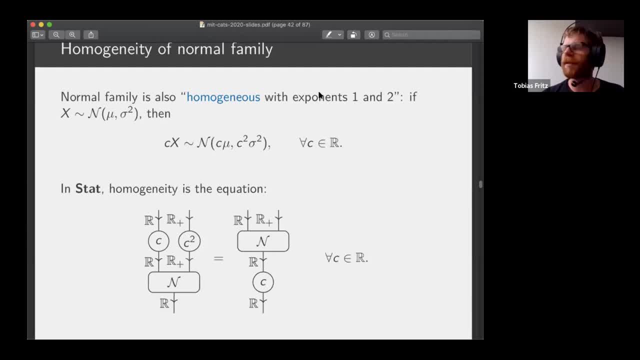 um, so if you did not consider, let's say, a vector space supply, then you can still have a prop, sort of prop for vector spaces, right? so then you would still have to vector space structure on, on, uh, on the objects in your theory, right? um so what if you consider just 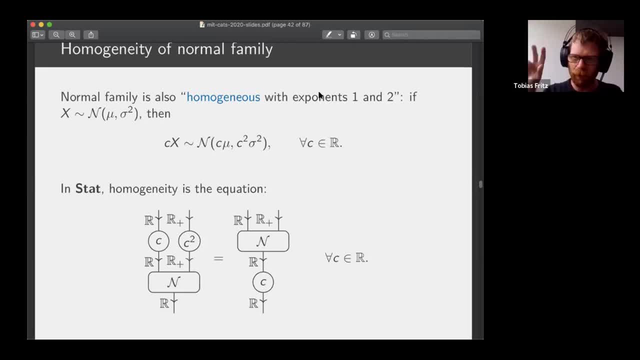 um, only common supply bumpers, then, for every such, or for every model of that theory, um, the target objects then will also acquire a vector space structure. yep, right, so what? what goes wrong? or does something go wrong? well, I guess the reason you might want to supply the vector space or other structure 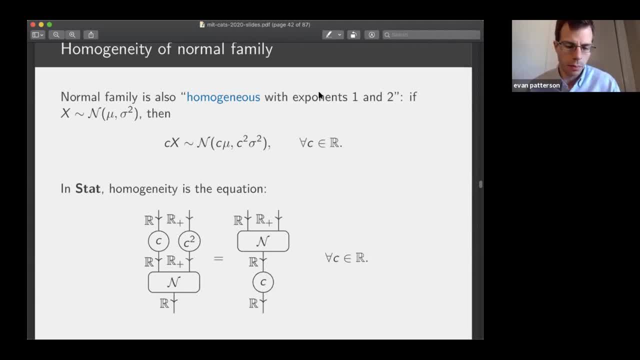 just like is the same reason that you would want, might like, to supply the cominoids as opposed to just it's that it ensures that when you take the structure of the vector space structure, you take monoidal products that those uh behave well right. so you would think that if you took 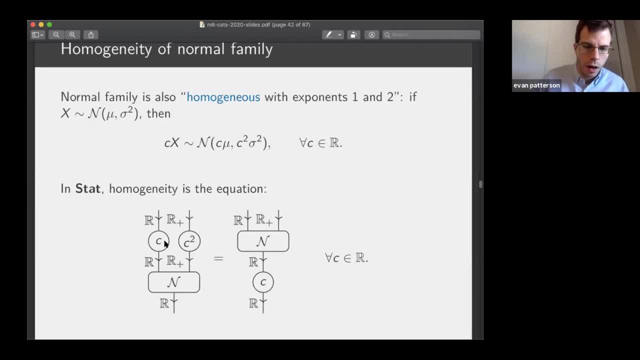 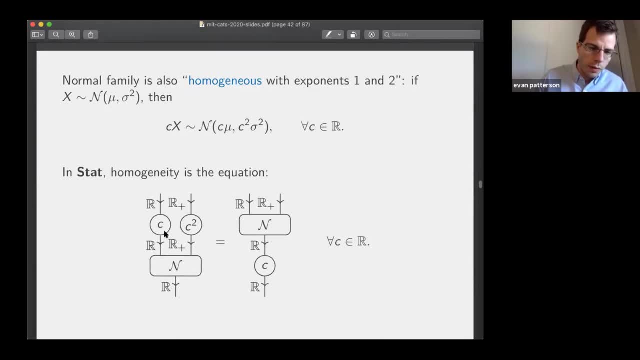 um. so actually we can. we can see it here, um like in this, in this very equation, actually, so like um, this space of r times r plus r, is a vector space object. this is a conical space object, so their product should be a conical space object. 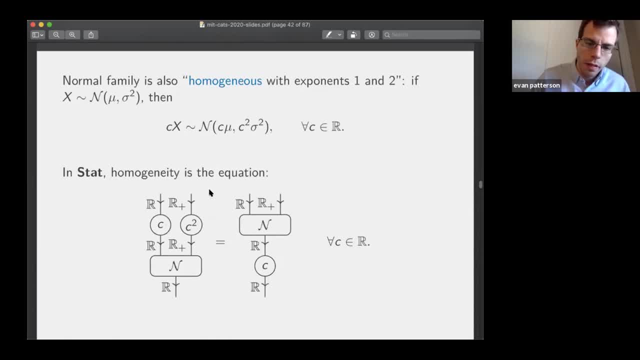 um, for example, and that those kinds of coherency conditions are what the notion of supply gives you. so so yeah, I mean, you're right, you could, you could, you can always, um, like, encode those props into your theory if you wanted to, but then you would no longer have this, this sort of coherence. 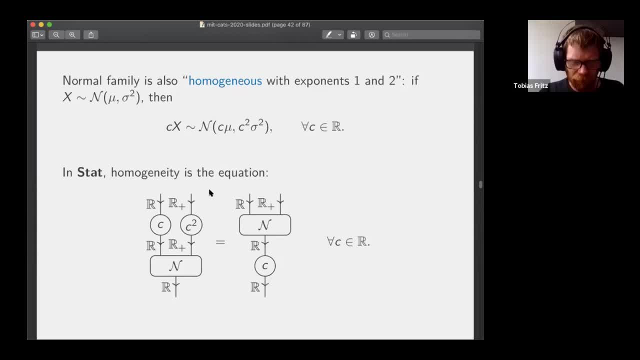 property. so yeah, well, wouldn't this be part of the defining equation? so if your theory, um, I think the main difference would be that, on the level of the target category, you would not start with the supplies already there, but they're sort of determined. the algebraic structures are undetermined by the model itself, right, but you would 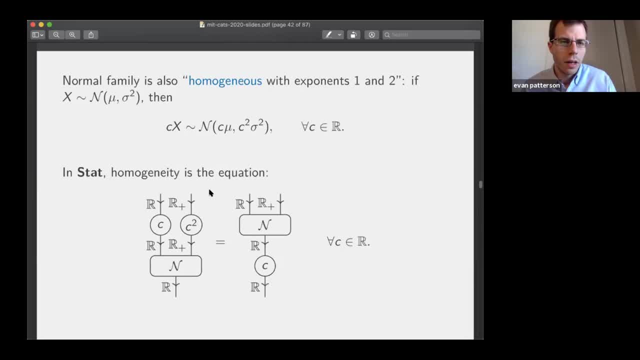 you would have to for basically for every. uh, yeah, I mean, I'm sure you could do it. I just think that you would then have to encode every time you used a product, object, like in your theory, like in your presentation. you would have to also encode the relevant props for those things, And then you should. 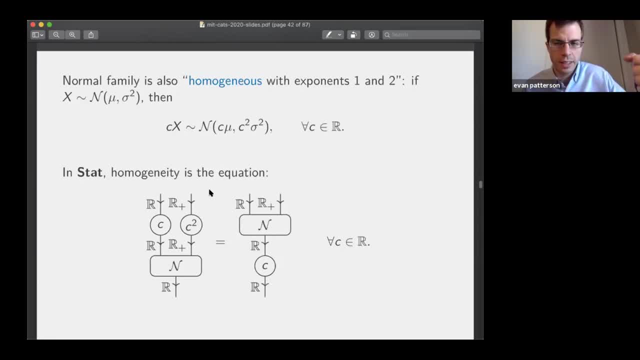 also probably put in the coherence axioms too while you're at it, And then at that point you've reproduced the definition of supply without actually using it. So I mean, yeah, so I guess my take is that it makes more sense to just if you're going to take that structure. 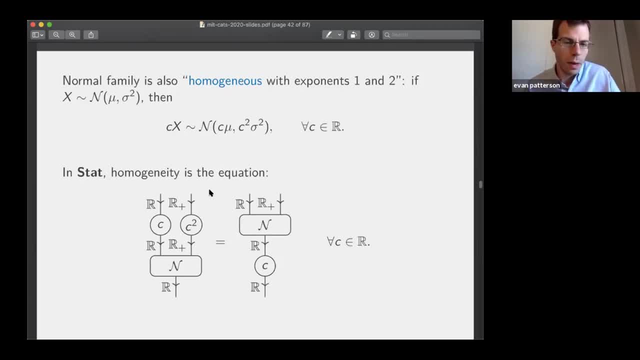 seriously, you should, you should do that, But then maybe maybe there I mean there are definitely, you know, like for certain kinds of models maybe you don't need it and you and you don't need to do that. But yeah, that's my take, I guess. Okay, Thanks. 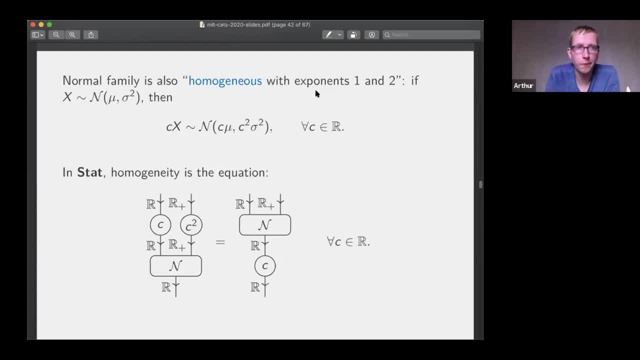 I was wondering what was known about Markov categories in terms of their constituting a notion of theory. So I assume you know they don't quite correspond to monads in the same way that the LeVere theory does, but maybe you could get almost as much, Has anybody? 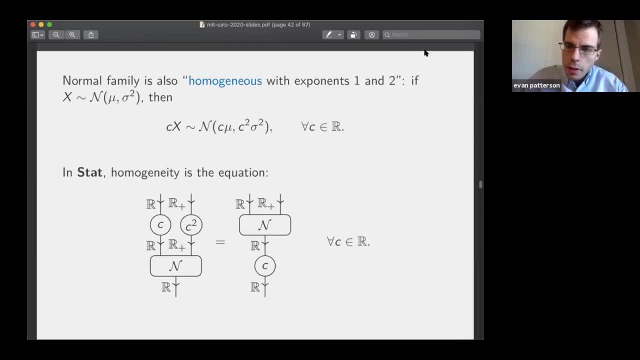 looked into those kinds of considerations. I don't know. I mean, Tobias, do you, do you know? No, but yeah, I, it's a very sounds like a really interesting question. So yeah, good question. One more question, unrelated, Evan, if I can, Any notions of closeness in the Markov categories? 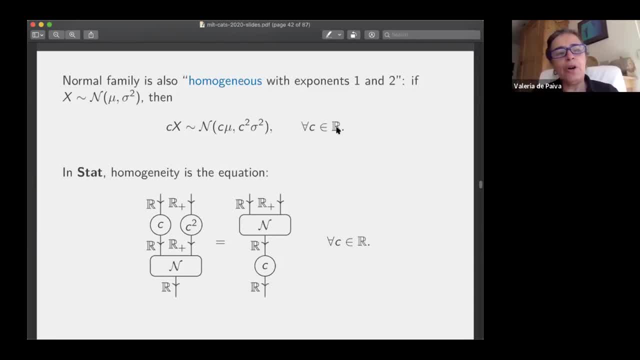 any notions of internal homes and stuff like that that we know of. So let's see. So I don't know about the case of Markov categories as well. I know that in the case of like just the category of measurable functions, it's not Cartesian closed, It's not. 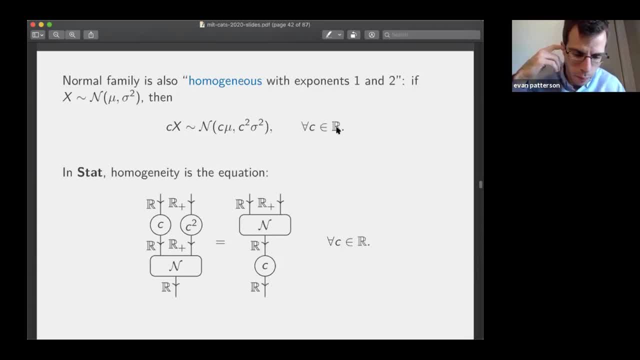 closed. And and and that has led people who study the semantics of probabilistic programming languages to introduce other categories that are: are better behaved in in our clothes, So things like it's like quasi Borel spaces and stuff like that. So in general, the, the and. 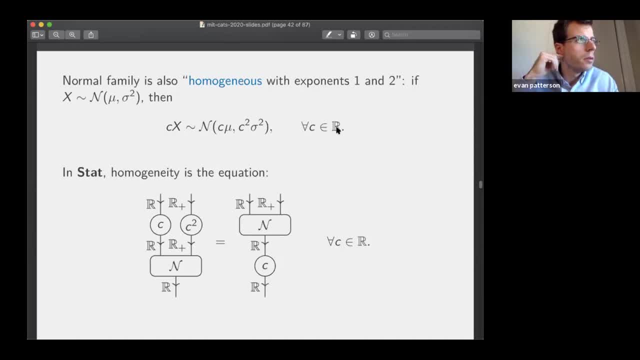 this was sort of implicit in my talk here- like just measurable stuff on its own with no farther assumptions, can be like very badly behaved. So usually in practice you put on you know some regularity conditions of some kind to to avoid that. Now in the case of like Markov kernels, 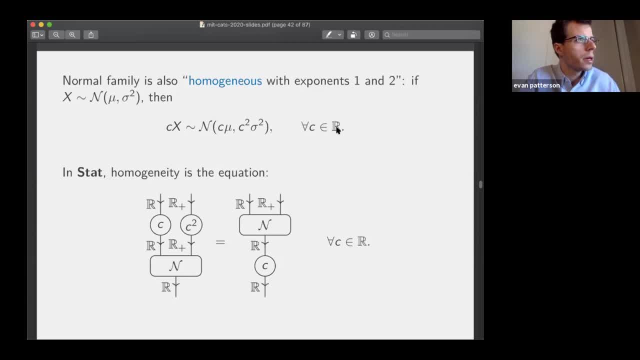 I don't think, I'm not aware of them being of people studying, whether they're closed or not. Again, I don't know if, Tobias, do you have any further thoughts on that or not? Yeah, So so those are typically. 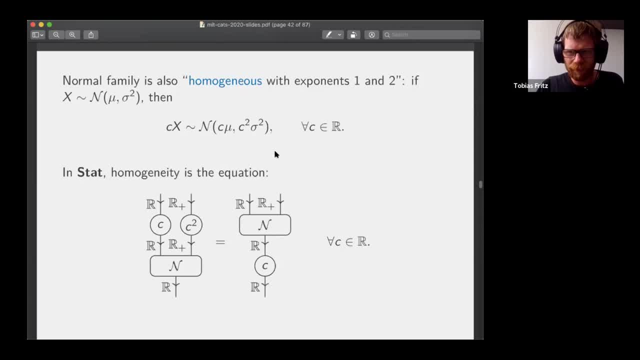 Kleisler categories. And so Kleisler categories are rarely monotone, closed, right, Except I don't know if a general statement, but neither. Yeah, A category of Markov kernels is certainly not monotone closed. But what has so much better? 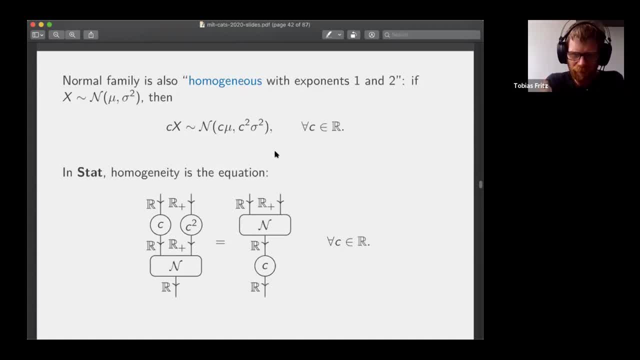 chance of being closed is in the Ellenberg-Moore category, Right? So all all the algebras, but there the problem is that then we no longer have the Co-Monnet structures. we can no longer copy. so. but maybe a way around that would be to work with the Ellenberg-Moore category, And so 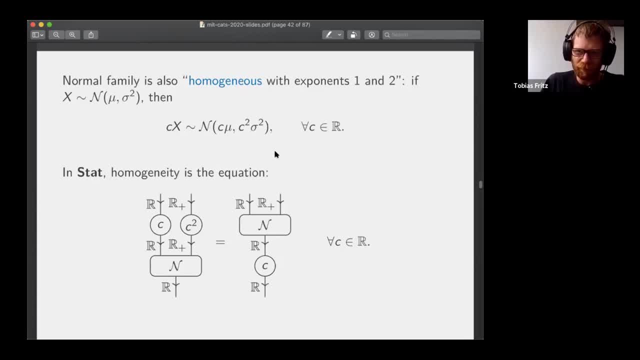 if you use the, the, the, the, the, the code, on that you know you can. you can just kind of, that's I, and then to supply only the three algebras with the Komono structure, which may fit well into. 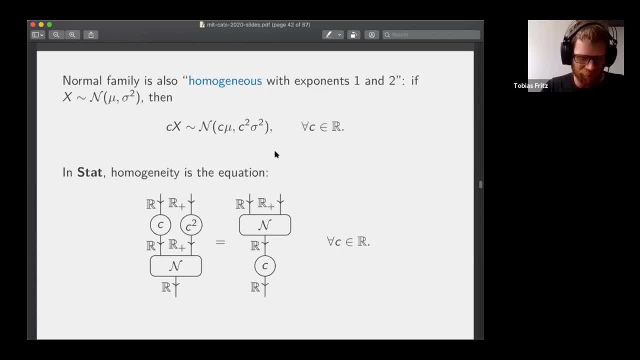 Evans' semi-latus of supplies framework. Does that help? Yeah, no, it does. I mean, of course, as you're saying, topological spaces in general have problems with closures, right, They are kind of. there is even a page in the lab which is called good topological spaces or well-behaved. 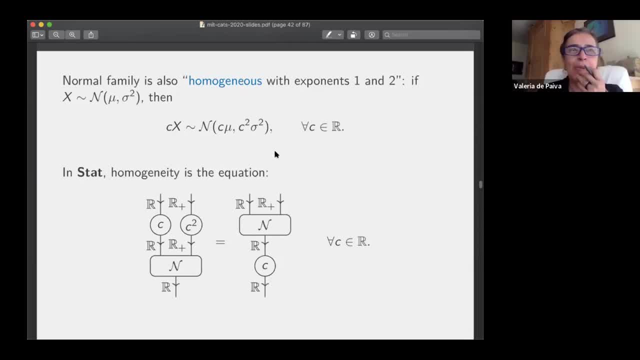 topological space or something. But normally, you know, normally one tries to see monoidal, closed structure kind of, whenever, as you say, we add the constraints to see if we can get it. And you know, the thought was that maybe there is, because you're kind of already doing this, very big constraints of 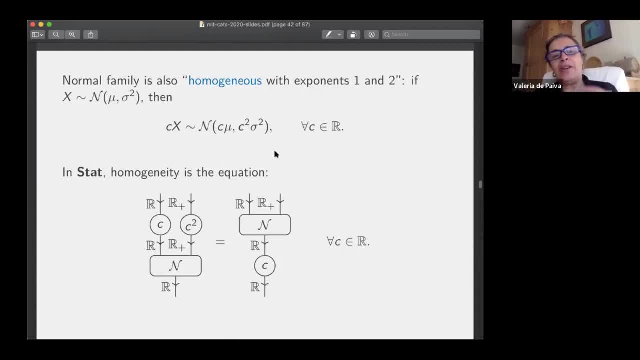 connecting these things to linearity. maybe there are kind of other constraints that come to mind. Yeah, it's worth investigating for sure. Thank you, Thanks, I mean, maybe one way that one can see that is that, let's say, a morph is in a Markov category from. 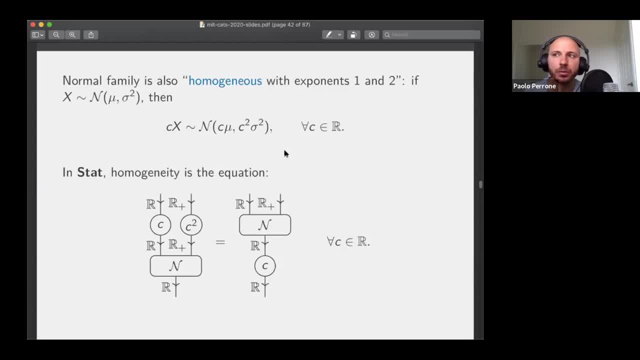 say a times b to a times b, And then a vector is in a random way. So if we wanted something like a Cartesian closure structure, a Markov category- even if it's linear or with extra structure, one would have to make sense of. 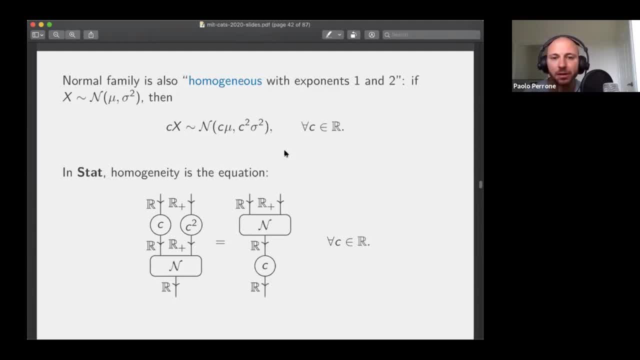 things that are, I mean, randomly parametrized. So Markov kernels from A to X, say, randomly parametrized by some B, and not just deterministically parametrized, And it's really hard to imagine those as corresponding to just Markov kernels on the Cartesian product or monoidal product. 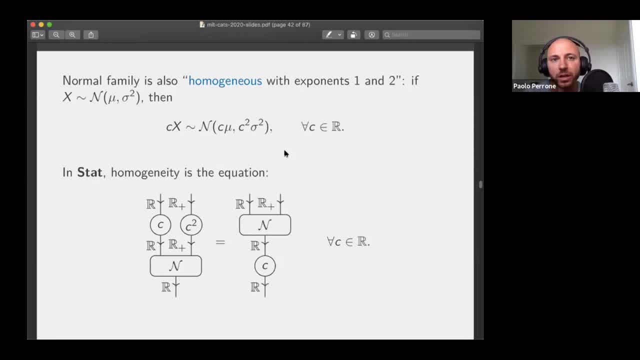 of some kind. This is true for I mean, this is true for like Kleisler categories. but more in general, If one thinks of the statistical meaning, it would be hard to see how one can get something like Cartesian closed structure. For sure there is a way to say some nice. 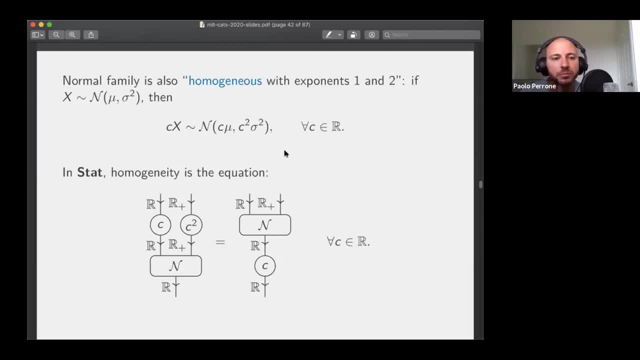 things about the morphisms. I mean, I'm thinking like quasi-barrel spaces, for example, for sure have very nice properties, but I don't think it's like a monoidal closure, or I mean not quite. So anyway, are there any more questions or comments or follow-ups?